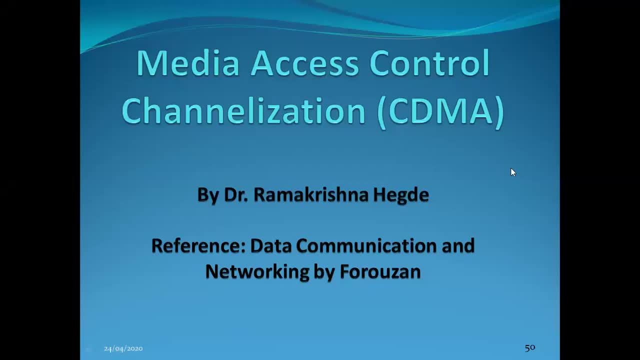 Hi everyone, my name is Dr Ramakrishna. Today let's discuss about one of the very important protocol comes under channelization. It's called CDMA. Here some of the material I've referred directly from a course on book It's called a data communication network, which I've mentioned. 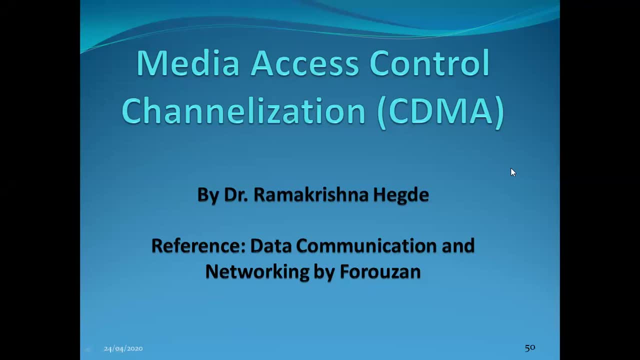 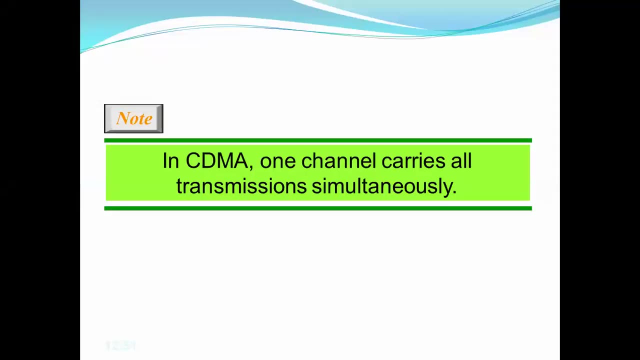 already in this particular slide. Now let's discuss about the protocol called CDMA. The CDMA is stands for Code Division, Multiple Access. In CDMA, what happens? One channel carries all the transmission simultaneously. Imagine you have multiple stations. In reality, you have. 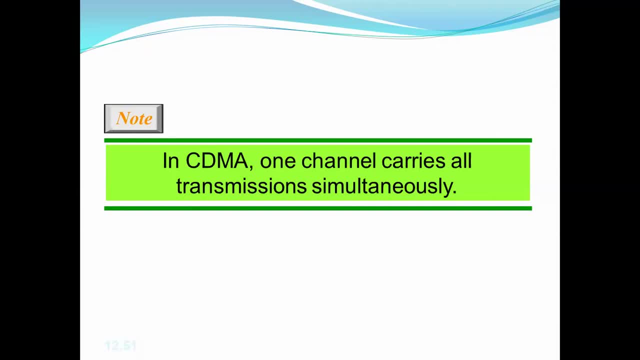 multiple stations. That multiple stations normally shares a single channel. Many stations normally share a single channel. In CDMA, what happens? The one channel carries all the transmission simultaneously. This is what normally happens. CDMA means communication with a different course. 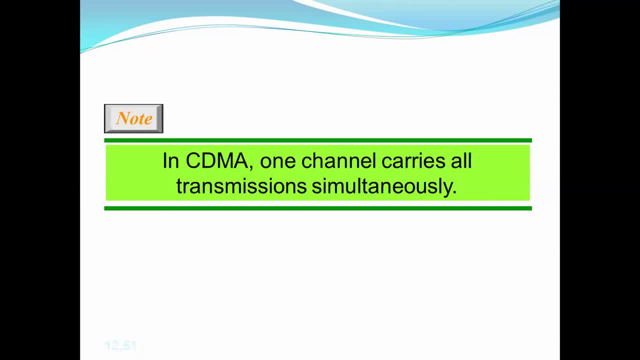 Name itself indicates Code Division. Multiple Access. That means CDMA means communication with a different course. That means every individual station will assign with a different course. here Every individual station is assigned with a different course. We can understand the CDMA by using some analogy. 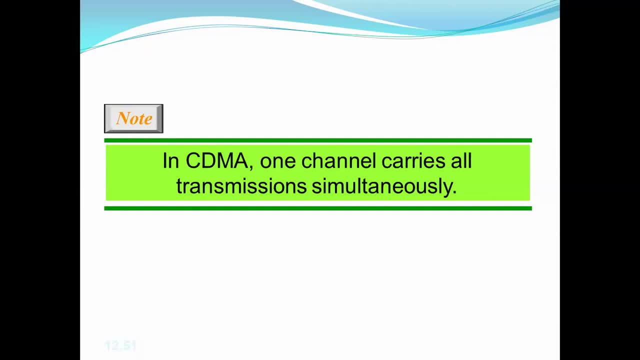 Here. let us imagine there are many people are sitting in a room. See, two people wants to communicate with each other. Let us imagine two people are talking with one of the language called English And other people will imagine other people will not understand English. Two people. 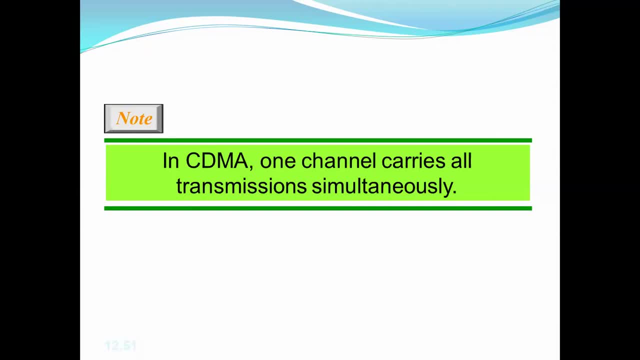 can able to speak in English. Now assume another two people are also talking in a different language. example: uh, in, maybe in hindi. maybe other people may not understand hindi, right, but only two people can able to understand hindi. so those two people will talk with each other like this: uh, you know? 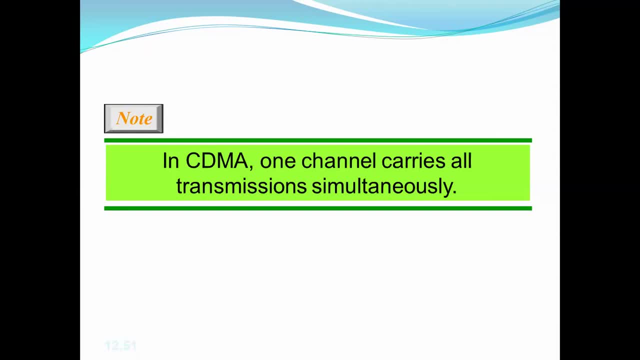 many people can able to communicate with each other in a certain code languages, certain codes, with the help of a code right. for example, what i've taken here in english is the code which maybe two people can able to communicate with a particular language called in english, but other. 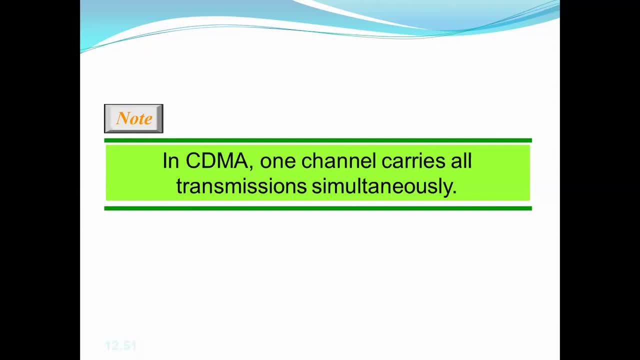 people will not understand that. other people will not understand english. that is why only two people can able to communicate with each other with a particular language called in english. right here what happens? a single channel, single channel. we can refer here the uh, the whole room space, whole room space. maybe we can refer as a single channel. right in that particular room there are 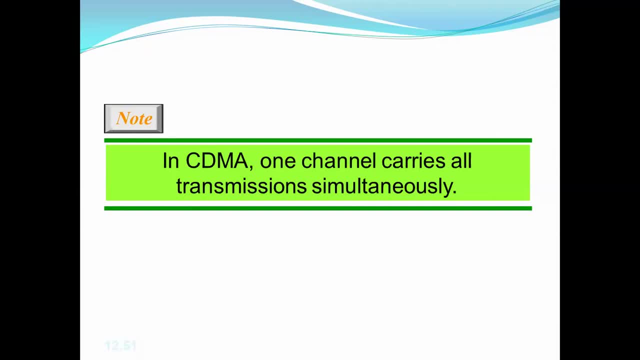 many people are sitting. right, many people are sitting, uh, sitting. that means you can, you can see the people, uh, maybe, uh, you know, uh connected as uh stations, different stations- right, many people are sitting in the particular room: right, the space of the room is we can take it as a single channel, right, uh, this is. 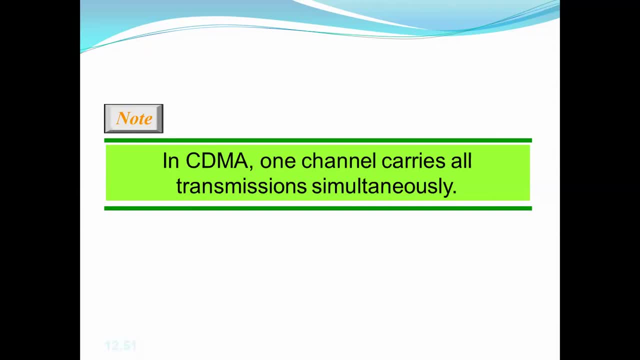 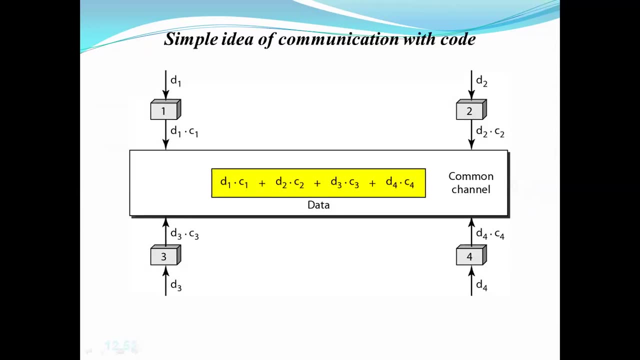 how we can understand, uh, about the cdma now, if we can refer this particular figure, if we can refer this particular figure. simple idea of data communication, maybe, how the communication exists, uh, in a single channel with the help of a code. now, uh, you can understand more. 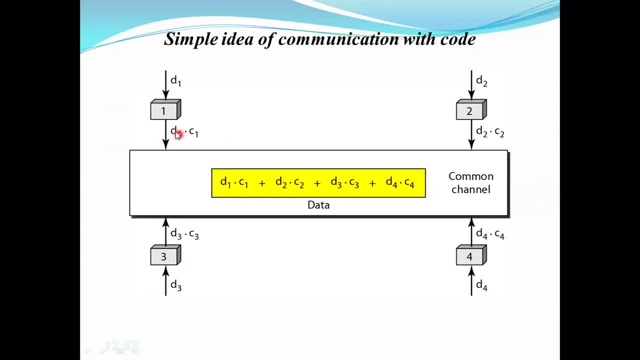 clearly. here you can understand more clearly. there are four stations, right uh: station one, station two, station three and station four. there are four stations. you can see here all the four stations are communicating over the single channel. this is what the single channel coming single channel right now, let us imagine, uh. so whatever the d1 we have represented, this is actually. 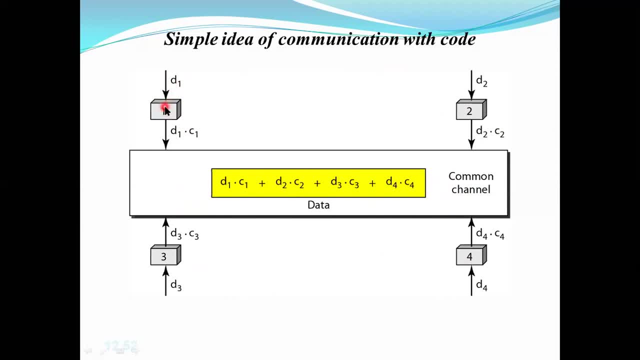 uh uh, station one is sending the data. the data of the station one: c1, what you referred, is the code 1. similarly, d2 is the data of the station 2. c2 is the code of the station 2. similarly, station 3 will have a data of d3 and code of c3. d4 is the station of data of the station 4. 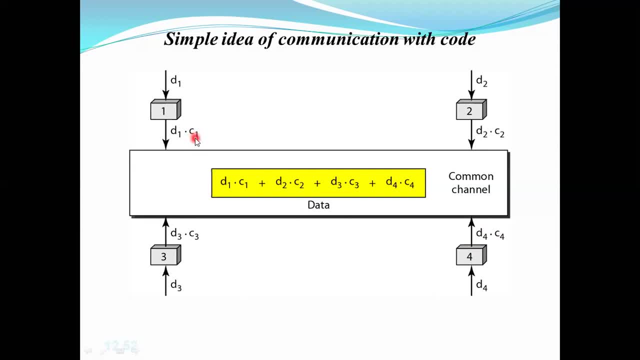 c4 is the code of the station 4.. now you can make out: c1, c2, c3, c4- all these codes are different here. that means every individual station is assigned with a different course. right, every individual station is assigned with a different course. now what happens? what the 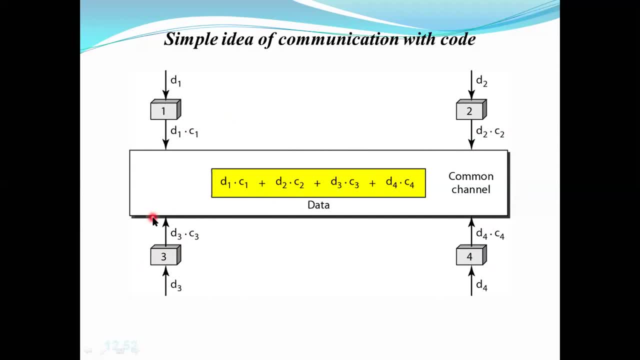 definition says here what the definition says: uh, in cdma one channel carries all the transmissions simultaneously. the word simultaneously means here you can see what happens. this is a single channel, right, the summation of all the data's, maybe all the station which sends the data, right. 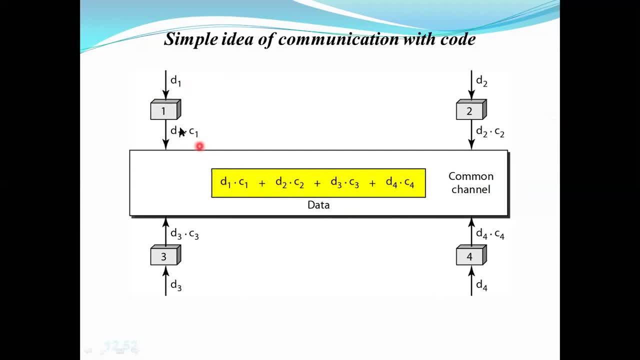 some of all the data's normally sense here. this case, you can see the station in in station one, right. uh, the data of the station one is multiplied with the code of the station one. this is actually forms one from the station one. similarly, at the station two, 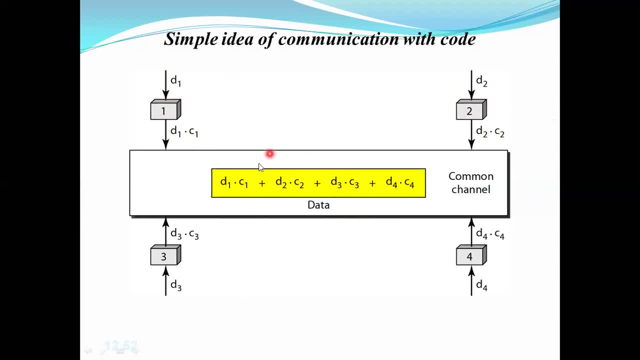 data of the station two is multiplied with code of that particular station. this is what comes here. then station three: data of the station three is multiplied with the code of station three. this is comes here, like, similarly it happens, the station four also. now what happened? the sum of 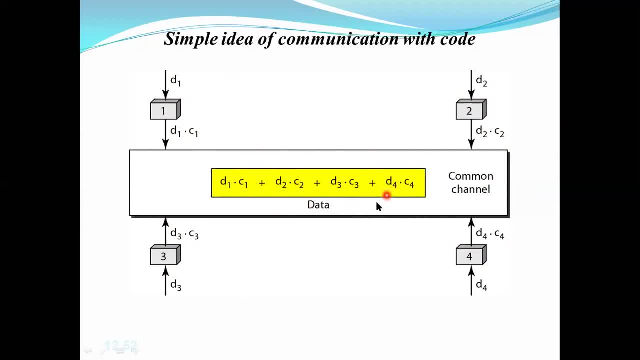 this, all this, uh, some sum of all these, actually transmitted over this particular channel. now this is become data. no right, uh right, this whole thing is become a data, whole thing has become a data and this is actually sent over the common channel. this is what normally happens in the 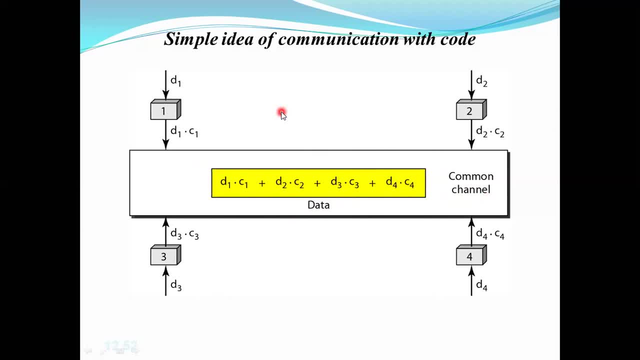 cdma, cdma, with the help of the different course now, uh, one of the very important thing you supposed to know when it comes to a code here, here. here we assume the code assigned to the station. should i have a following properties: right, whatever the code is supposed to be assigned to individual station, right, should have the 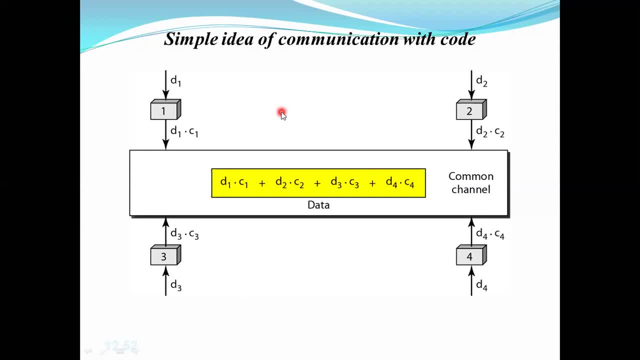 following should have following properties. first property is that, uh, if multiply each station, okay, if multiply each station by another, result should be zero. if multiply, let us imagine, uh, station one and station two, multiply the code i'm talking about related to code here, code of station one and code of station two. if you multiply, the result should be zero, that there is a first. 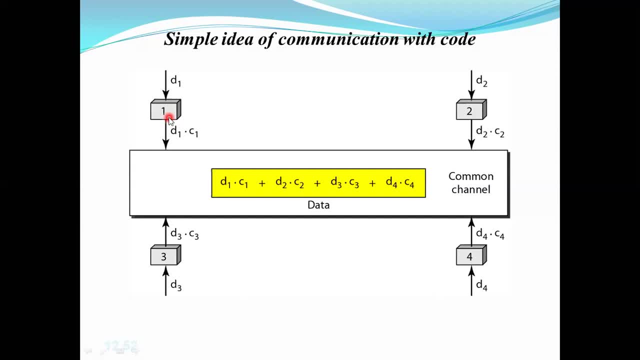 property right now. second property is: if you multiply each code by itself. if multiply each code by itself, the result should be four. let us take an example of station one which is having a code of c1. now c1 is multiplied by itself, that is, c1 multiplied by c1. the result should be four. 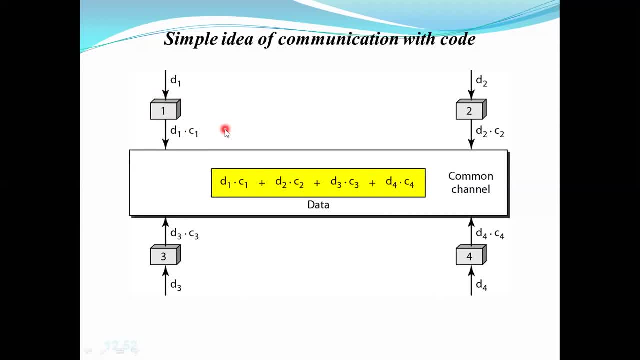 results should be four. this is the second property of the code. you need to remember that. okay, we need to assume these two properties when you assign a code to the stations. now, uh, one more very important thing you supposed to know is that suppose, uh see, there are four stations are communicating over the. 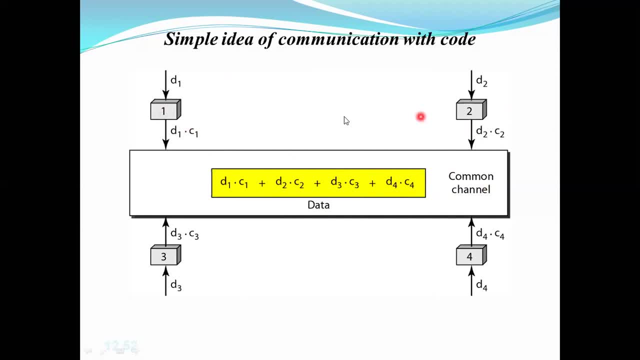 common channel here, but imagine there are only two stations. wants to talk to each other station one to each other. station 2 is hearing from station 1. station 2 wants to hear from the station 1. what is actually happens here? this case, what happens now? the station 2 right? uh, this case. 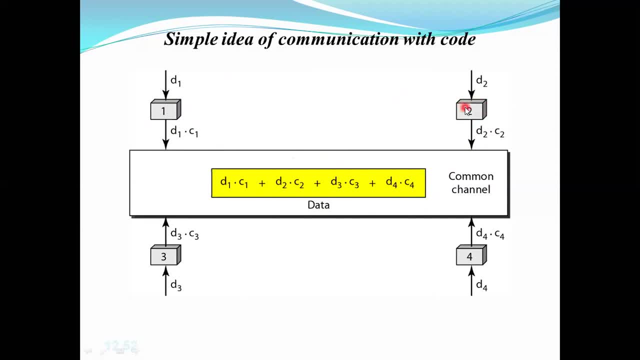 what happened? the station 2 multiply its data with the code sent by station 1. okay, with the code sent by the station one. right now, the station two- what actually does now the station two, what actually does- should have to the divide the result by 4 to get the data from the station one. 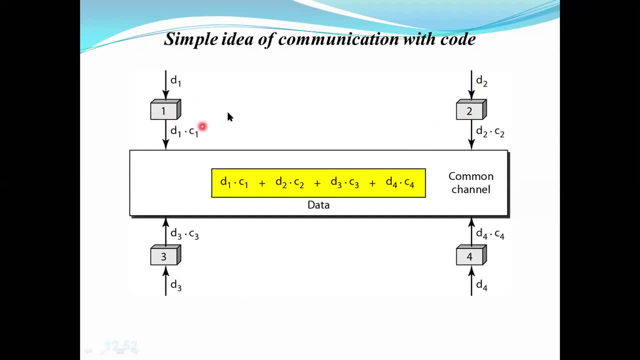 whatever the result you got it. when you multiply with d2 with the code sent by station one, whatever the result you're going to get it, that result, unit 2- you have to divide it by a particular value: 4 divided by 4, then you will get an exact data which is sent by the station d1. now the station d2. 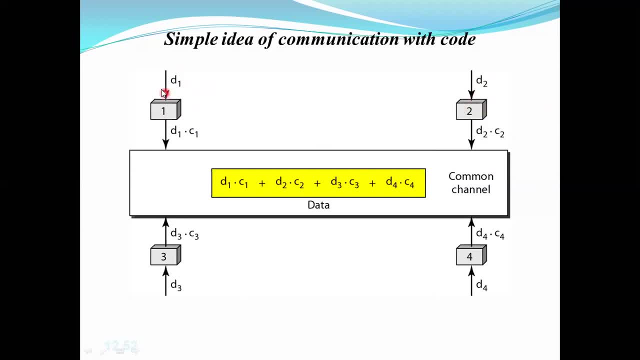 can able to get the data. what is actually the original data? i can able to get it from the data which is sent by the station one. okay, uh, this is how normally happens when the communication uh exists between two uh different stations, uh different station in this particular uh arrangement here. now uh another very important. 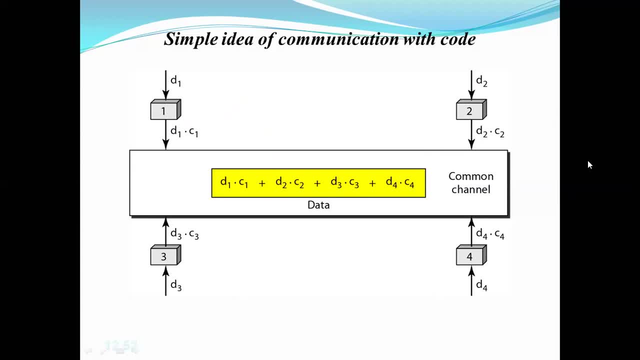 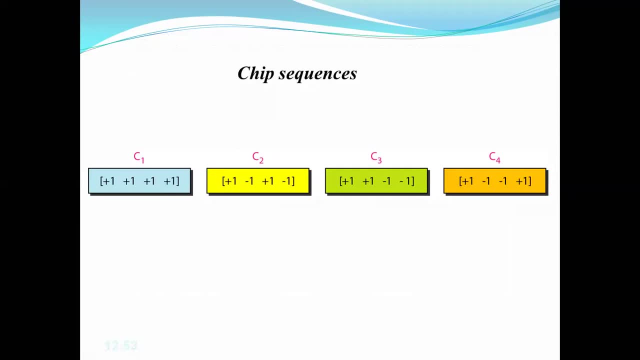 uh thing you need to discuss here is called. call it as chip sequence now, what is actually meaning of chips? so you're supposed to know the meaning of chips first now? uh, chip is nothing, but each station is assigned with a code right. each station is assigned with a unique code right. 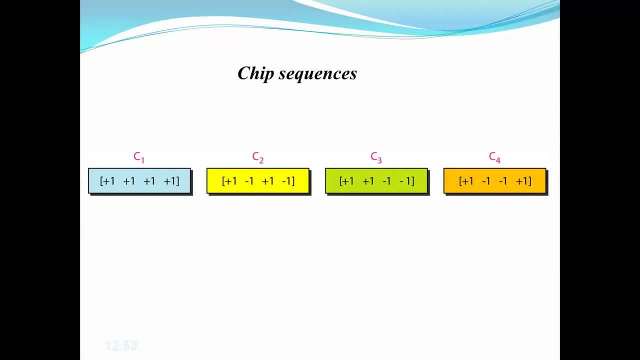 each station is assigned with a code. code which is the sequence of numbers. right, code is nothing but a sequence of numbers. that is actually called it as a chips. right, each station is assigned with a code, which is the sequence of numbers. normally call it as chips, normally call it as a chip. chip here, right? 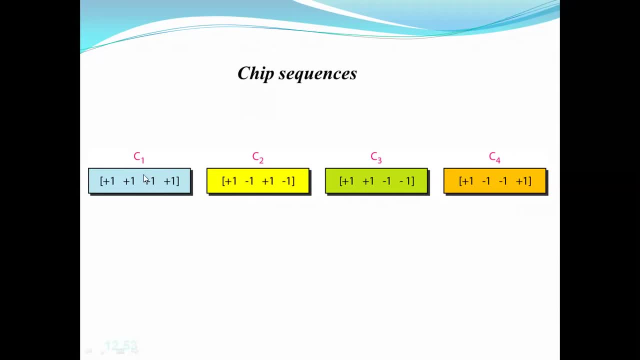 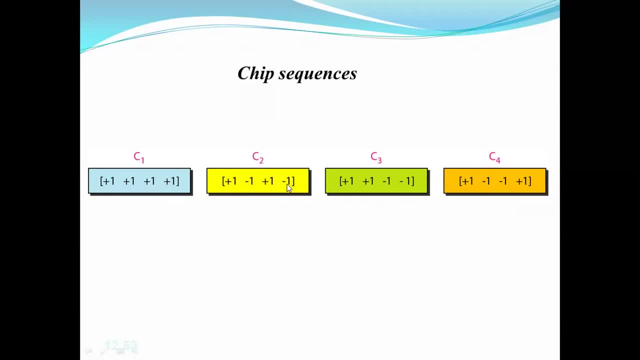 you have another sequence called plus one minus one. plus one minus one. now, what is this? plus one minus one? so whenever the station is sending the data, uh, sending the data, uh as one, sending the data as one. okay, now that is actually we, we actually call it. 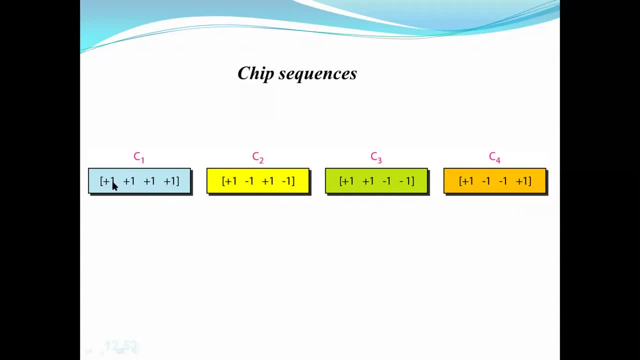 as one. whenever the day of the that is actually called it as plus one. whenever the station is sending the uh data value zero, that we are representing as minus one, that we are representing as minus one. suppose the station is not sending any data, then the value can be represented: the uh, the value which is in the sequence you can write. 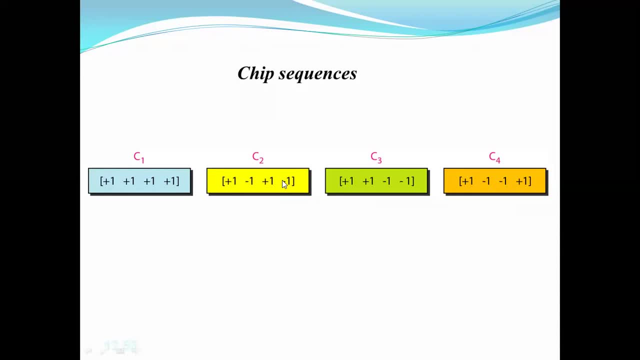 write it as a zero. write it as zero, right? suppose station wants to send the data as one, then the number you are going to represent in the sequence is plus one. suppose the station wants to send the data, sending the data as zero, right, the number you are representing in the sequence? 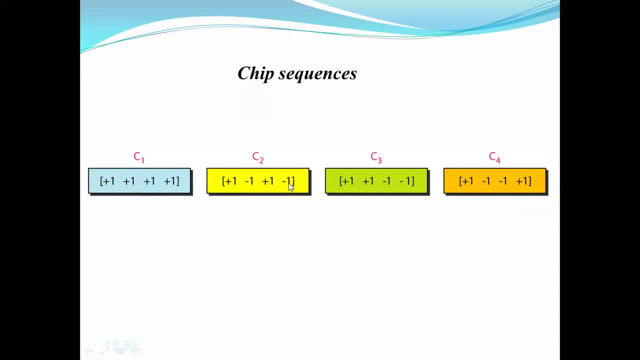 is minus one here. minus one actually represents the station is sending zero, plus one represent the station is sending one. suppose if zero comes, suppose there is no zero in this particular sequence. suppose zero comes in the sequence, that means the particular station is not sending any data. right, that is actually meaning here. now this is about the chips. 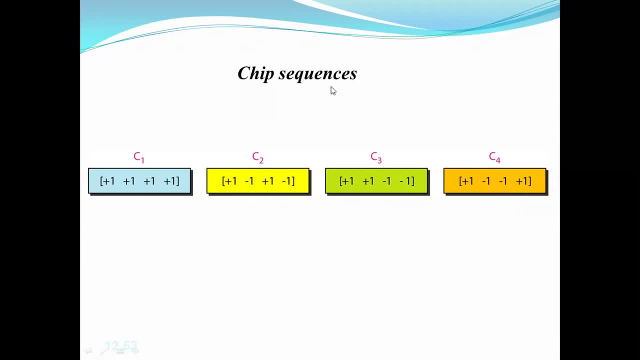 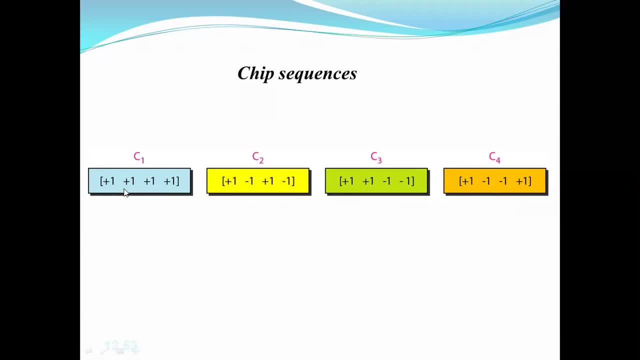 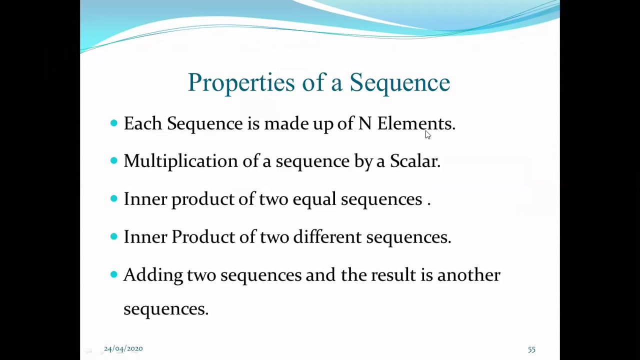 need to discuss here. the first property of the sequence is: each sequence is made up of N elements. okay, see, this is actually property of a sequence here. property of his sequences: each sequence is made of of n elements. okay, each sequence is made up of n elements, n elements. now, second property: 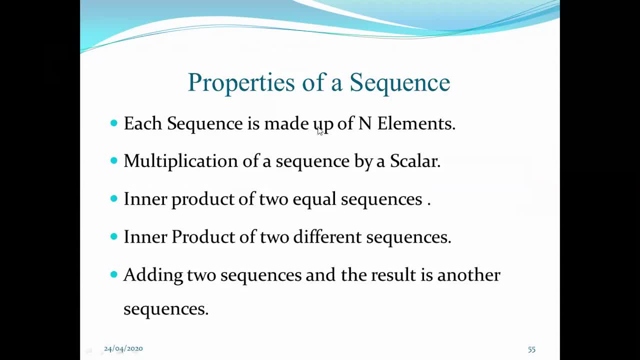 here, n actually represents the number of stations. each sequence is made up of n elements. so whatever n you are going to represent is the nothing but a number of stations. okay, now uh. second property: uh is multiplication of a sequence by a scalar value, the scalar value. we can take any scalar value, for example. 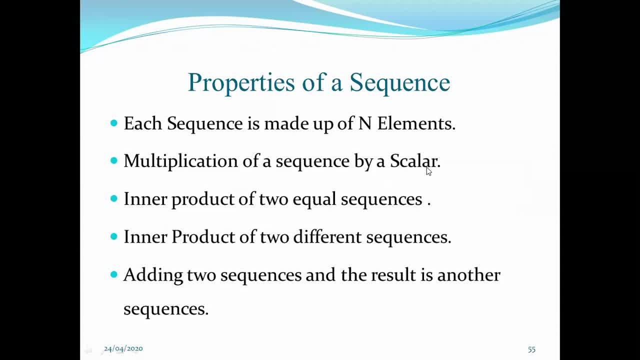 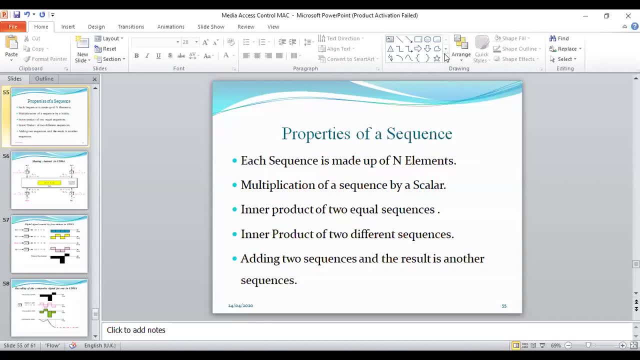 if we can take scalar value as 2, we'll we'll see how this. you know multiplication of the scalar value here is 2, then we can able to understand by calculating the number of stations, and we have just one. let's just wait for two minutes. 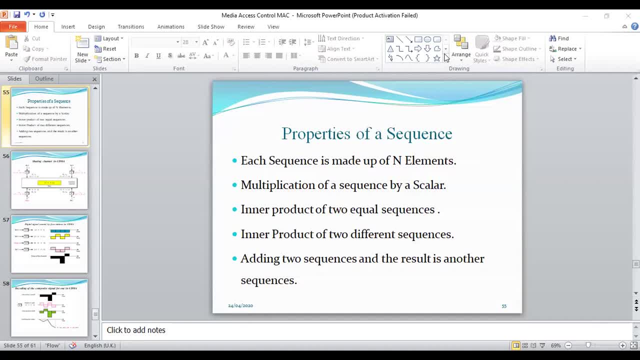 just to wait for two minutes, and i think we can able to understand here. we just wait for two minutes. so, in this case, what happens? let us imagine, right, uh, multiplication of a sequence by a scalar. let us imagine two, two. you need to multiply, two multiplied by, okay, two multiplied by. you take one of the sequences, you take, you take one of the. 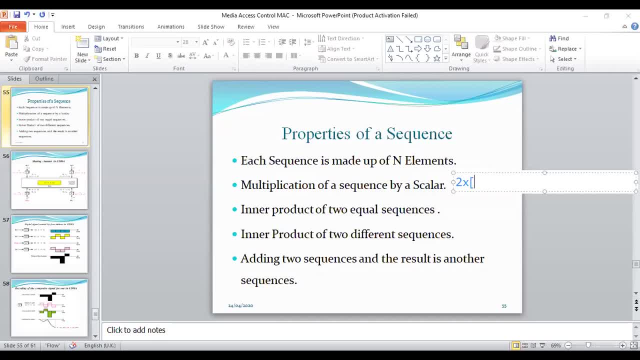 sequences: maybe plus one, okay, take as plus one. then another one is plus one, right? another one is: maybe you can take it as minus one, then another one. you take it as minus one. now this case, what happens? what is actually a result of this? the result of this is supposed to be what? 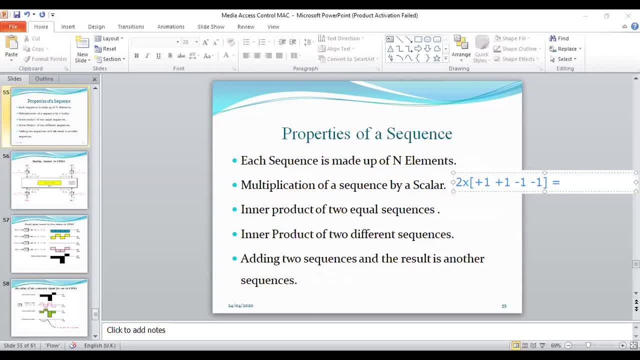 is equal to what result of this is supposed to be. you will get another sequence, another sequence, right. the result, sequence, resulted, sequences, what happens? this is a plus two comma plus two, right, not a comma here. plus two, then you have, then you have. what is the next one? minus two. then you have minus two, right, then you have a minus two. 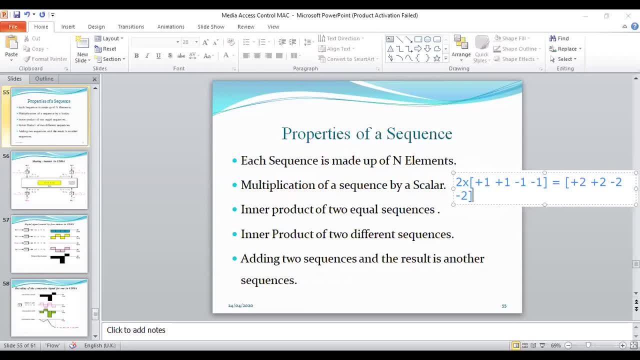 this is actually uh meaning of multiplication of a sequence by a scalar value right. that means this two is a scalar value right. this two should be multiplied with every element in the sequence. there are four element in the sequence: right plus one plus one minus one minus one. this scalar value. 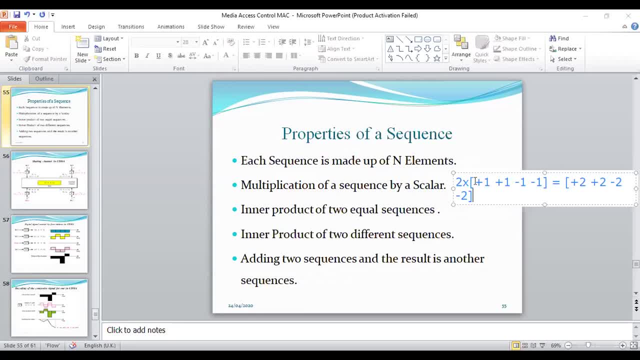 should be multiplied with every element in the sequence, every element in the sequence. that's what we have done here. multiply with every element in the sequence. this is what we we got the. this is what we have got it right. multiplication of the sequence here: right, this is the uh. this what the second one. now let us uh take it as a third one. 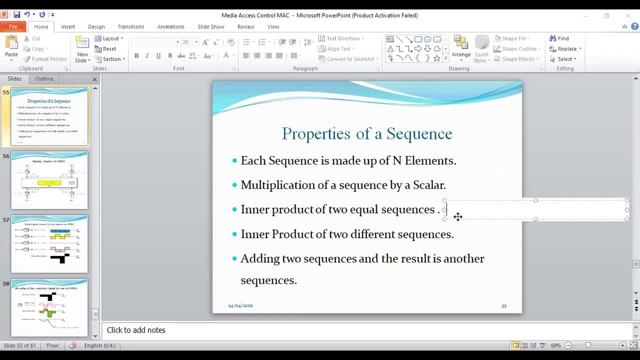 let us take it as the third one, that is, the inner product of, uh, two equal sequences. inner product of two equal sequences? that will likely so the inner product of the twoâl sequences. l you need to Take A take two equal sequences. here it should be two equals equal sequence. let us take what is the. 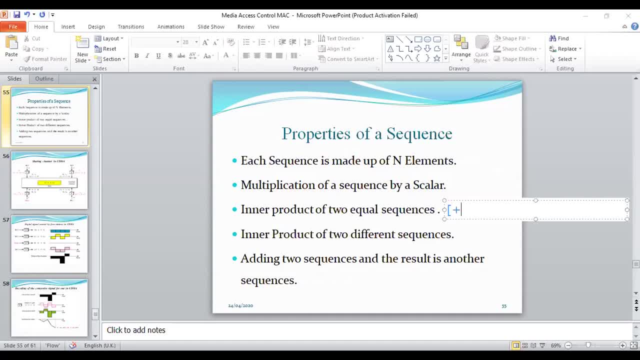 meaning of two equal sequence here. let us take first value as plus one, okay. then you have another, one is a plus one. then you have a minus one, right, minus one. you take, uh say, uh, minus one. you take one more value as a minus one, okay, minus one. then you need to multiply it, uh, what is that equal? 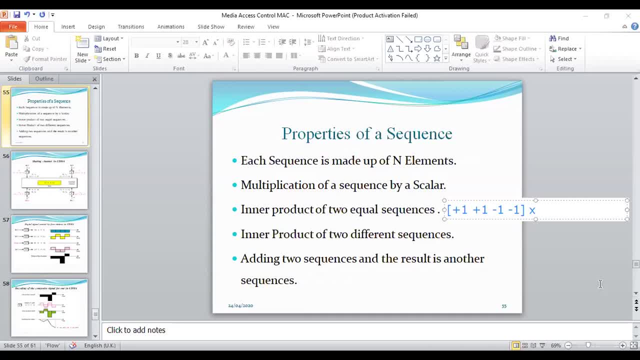 sequence. equal sequence in the sense should have a similar value. same value should be there here also. equal sequence, right? that means you should have. what is that? uh, plus one, then you have plus one, then you have minus one, then you have minus one, minus one, right? you need to multiply this. 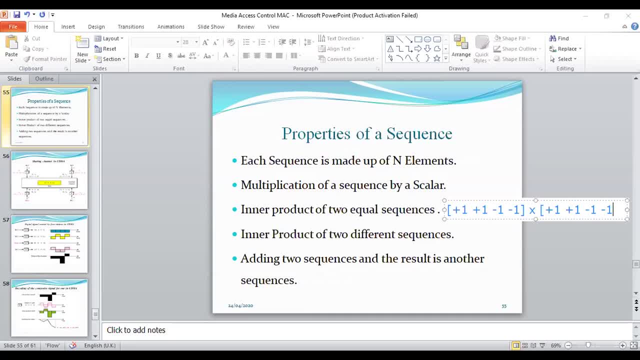 you need to multiply this now. when you multiply this, when you multiply this, what is the result here? what is the result? you are going to get it here, right, right, you need to. uh, what is the result supposed to be? so here, plus one, plus one, what is what is? 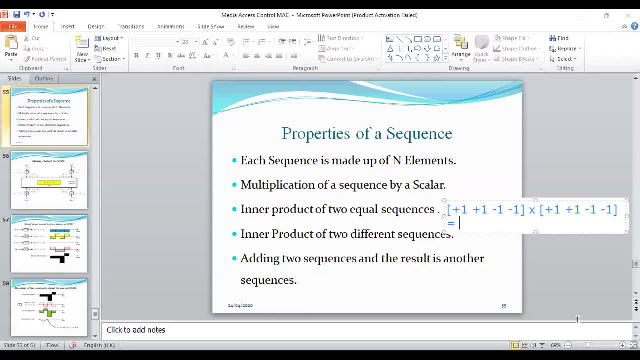 the result supposed to be. it should be one. right, it is one, multiple is one. then again, multiply with this is actually plus, okay, plus, then one and one again. you'll get a plus one here, right, then again: multiply minus one, minus one. if you multiply these two, what happens? it comes again to one. 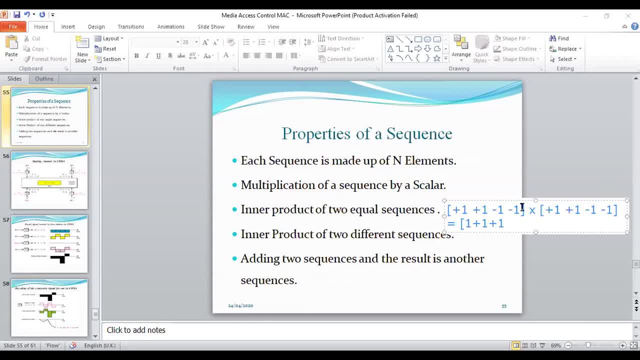 we'll get again plus one, it's again plus one, then again minus one, minus one and minus one. if you multiply these two, you'll get again plus one, you get a plus one, right, right, and this is uh, minus one and you have a minus one here. 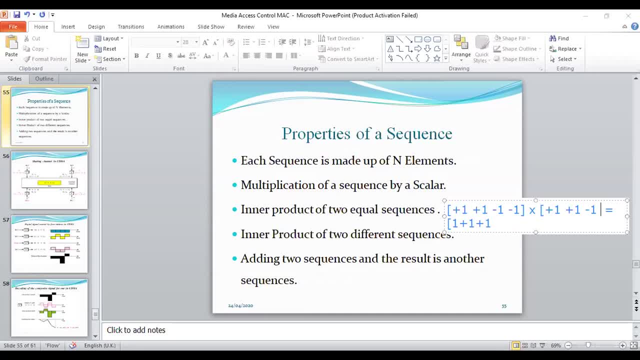 minus one. once this the result is, you know, equal, all right plus one. then you get a plus one right, zero, right the result. what is supposed to get? it is what? here is the plus 1, now, right, here is a plus 1. this is what the resultant, that means, inner product of two equal. 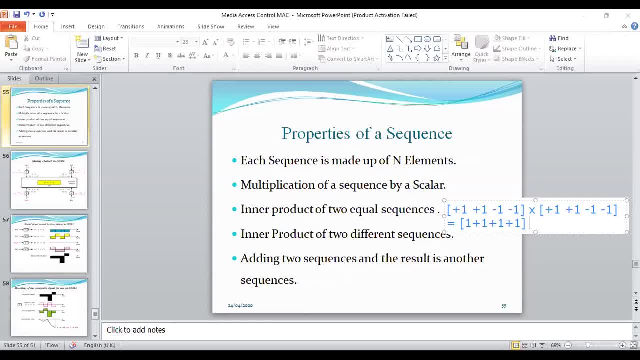 sequences, whatever you are going to get it here. what is the value of this? this is equal to. this is equal to what? equal to 4? the value of this is equal to 4. well up, this is equal to 4. now you can see this right. inner product of the two. 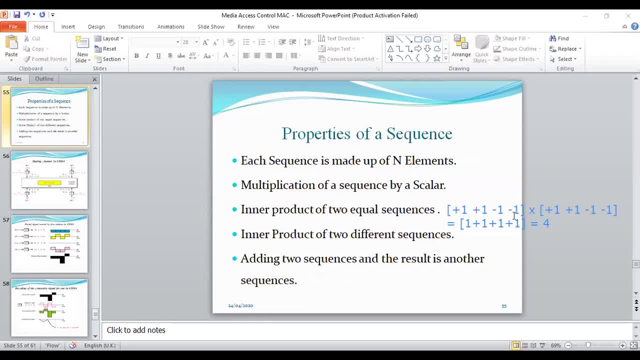 equal sequences. this is one of the sequence you can see. this is one of the sequence right? this is one of the sequence. one of the sequence. this is the second sequence. you need to multiply by these two. what is the value? you're going to get it as a 4. this is the third property of a sequence, inner product of. 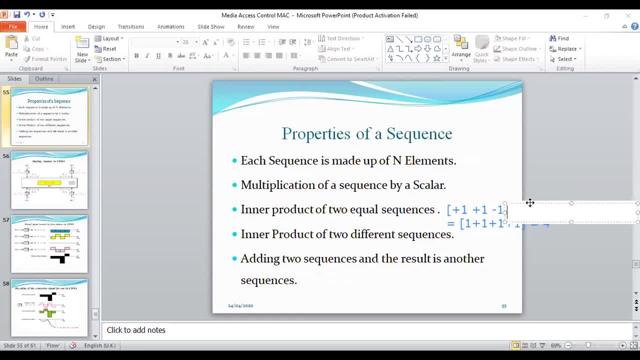 two equal sequences. okay to equal sequences, right, you, you now. so we'll come back to the. what is that? another one is a very important now, so we'll come back to the. what is that? another one is a very important one. another important one. fourth property is that inner product of two. 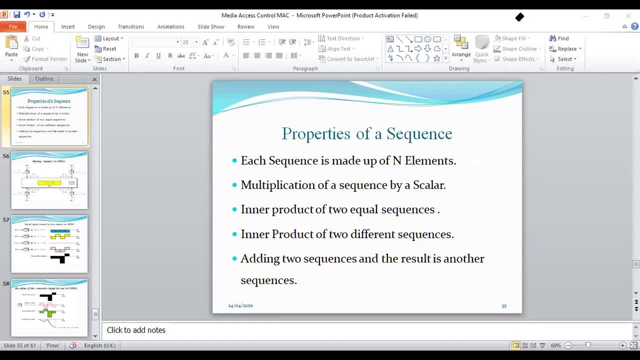 another important one. fourth property is that inner product of two different sequences. now, what is the different sequences now? what is the different sequences now? what is the meaning of you know inner product of two. meaning of you know inner product of two, meaning of you know inner product of two different sequences? we'll see this. what? 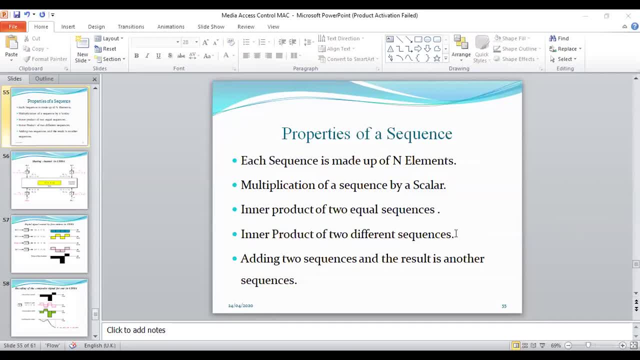 different sequences? we'll see this. what different sequences? we'll see this. what is the inner product of two different? is the inner product of two different? is the inner product of two different sequences? okay, two different sequences, the sequences. okay, two different sequences, the sequences. okay. two different sequences. the first sequence, let us take it as a. 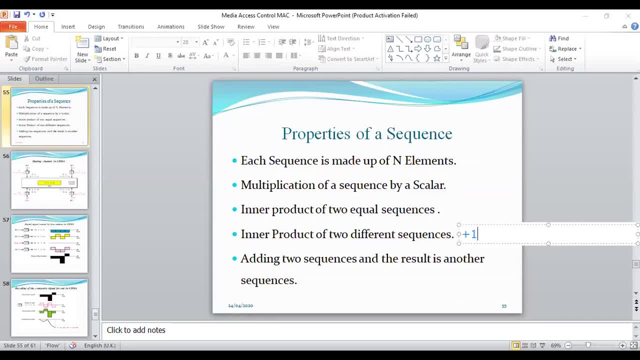 first sequence. let us take it as a first sequence. let us take it as a? uh first sequence as plus one. uh, first sequence as plus one. uh, first sequence as plus one. then you have another one is a plus one, then you have another one is a plus one. 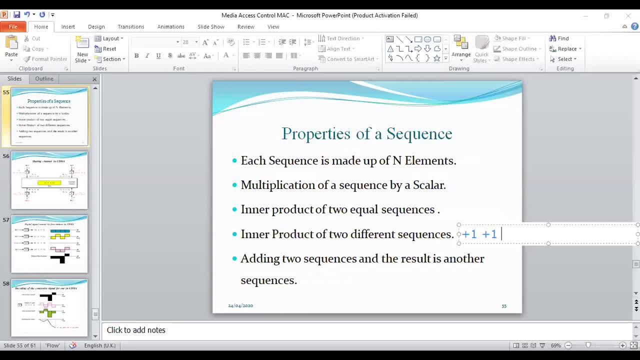 then you have another. one is a plus, one will be taken. then you have minus one you have taken. another sequence is minus you have taken. another sequence is minus you have taken. another sequence is minus one you have taken as another sequence one you have taken as another sequence. 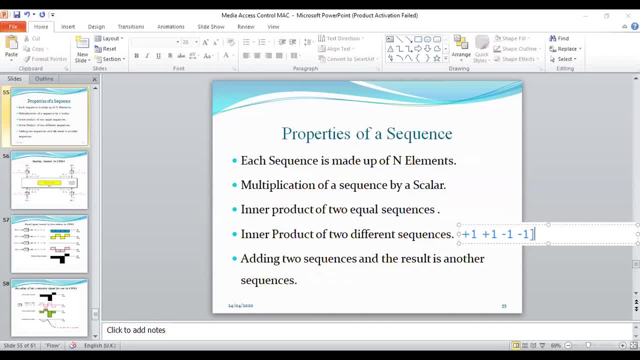 one you have taken as another sequence. another element as minus one right, another element as minus one right, another element as minus one right. this is the first sequence we have taken. this is the first sequence we have taken. this is the first sequence we have taken it it. 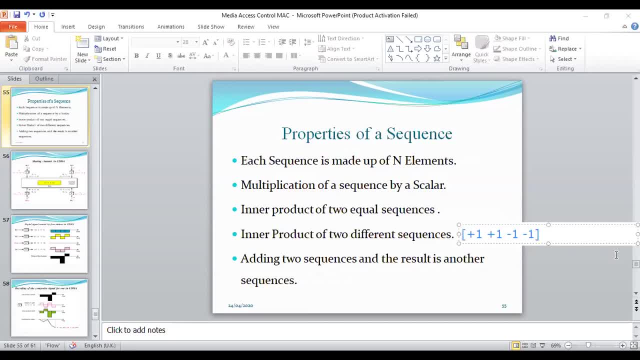 it. this is the first sequence. okay, then you. this is the first sequence. okay, then you. this is the first sequence. okay, then you need to multiply with the second sequence. need to multiply with the second sequence. need to multiply with the second sequence? what is the second sequence supposed to be? 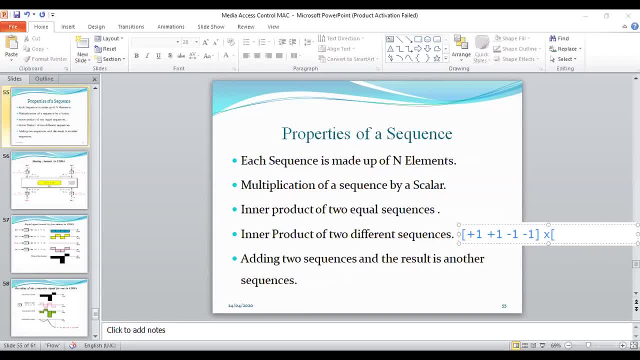 what is the second sequence supposed to be? what is the second sequence supposed to be? second sequence supposed to be plus one. second sequence supposed to be plus one. second sequence supposed to be plus one. let us take it as plus one. let us take it as plus one. 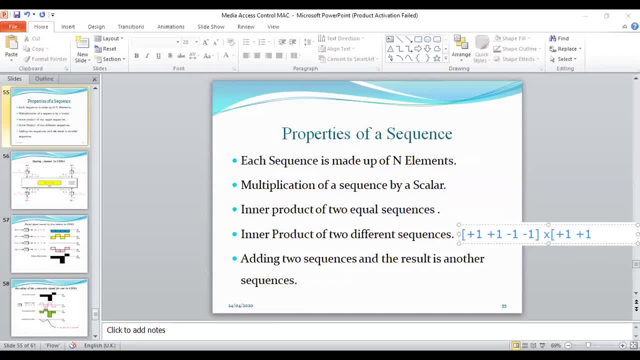 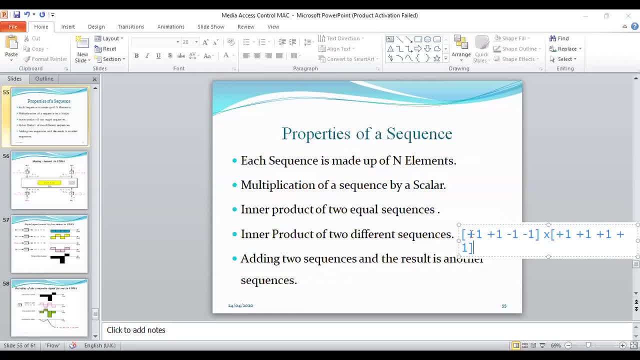 right again, we have taken plus one. now. right again, we have taken plus one. now, right again, we have taken plus one. now, these two are different sequence right. these two are different sequence right. these two are different sequence right. this is the first sequence is the second. this is the first sequence is the second. 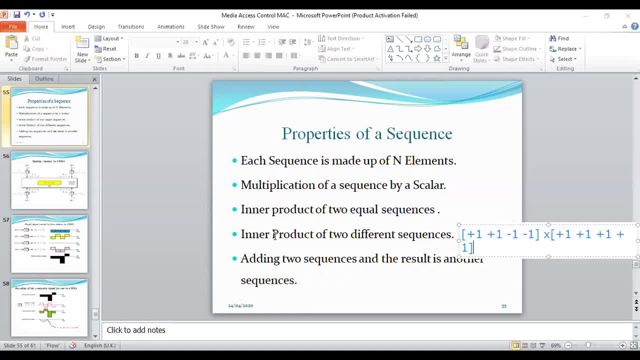 this is the first sequence, is the second sequence. first sequence is different for sequence first. sequence is different for sequence first. sequence is different for the second sequence. that is actually the second sequence, that is actually the second sequence. that is actually meaning, meaning, meaning inner product of two different sequences. 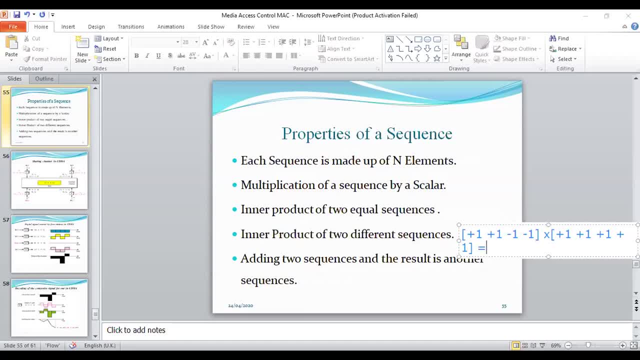 inner product of two different sequences. inner product of two different sequences. what is actually value you're supposed to. what is actually value you're supposed to. what is actually value you're supposed to get it here. what is the value? get it here. what is the value? get it here. what is the value you're going to get it, you'll get a one. you're going to get it. you'll get a one. you're going to get it. you'll get a one more sequence right. that means what is more sequence right. that means what is more sequence right. that means what is the value. you're going to get it. 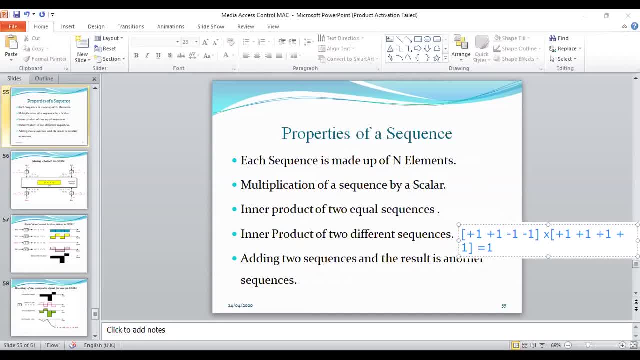 the value you're going to get it: one multiplied by one. how much you are multiplied by one, how much you are multiplied by one, how much you are going to get one right going to get one right. going to get one right, one then one, you will get it right. 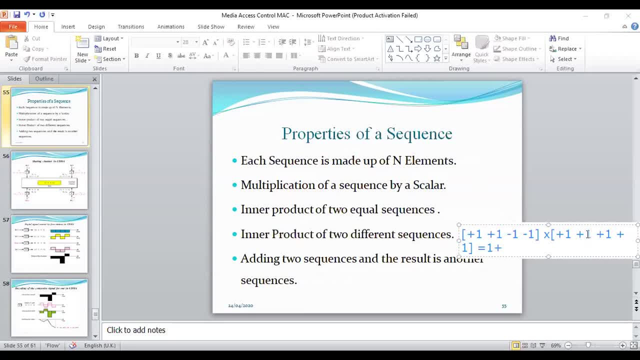 one then one, you will get it right. one then one, you will get it right. then plus one multiplied by one again, then plus one multiplied by one again, then plus one multiplied by one again. you are going to get plus one here. you are going to get plus one here. 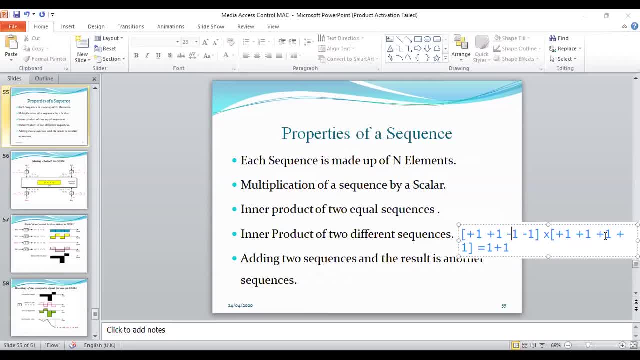 you are going to get plus one here, then minus one, then minus one, then minus one, minus one multiplied by plus one. what is minus one multiplied by plus one? what is minus one multiplied by plus one? what is the result supposed to be? the result supposed to be. 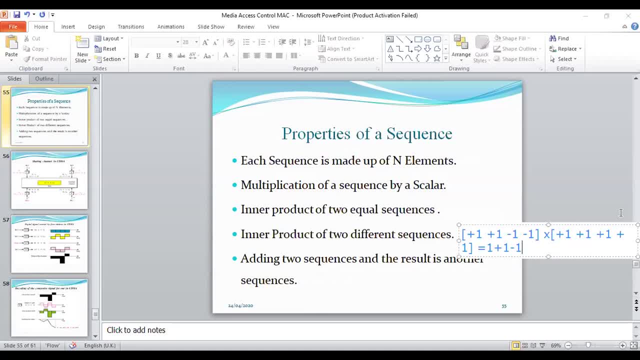 the result supposed to be is supposed to be minus minus one. is supposed to be minus minus one. is supposed to be minus minus one. then again last element in the sequence, then again last element in the sequence, then again last element in the sequence minus one multiplied by. 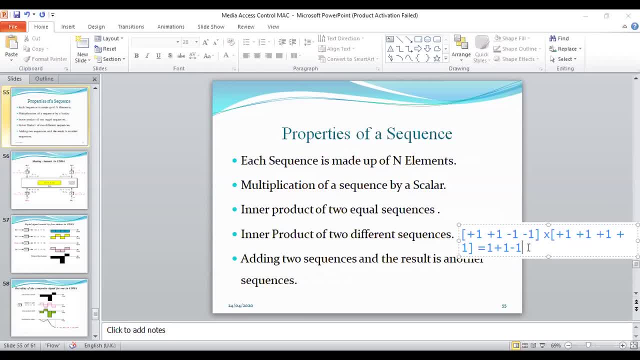 minus one multiplied by minus one. multiplied by plus one minus one multiplied by plus one plus one minus one. multiplied by plus one plus one minus one multiplied by plus one, what is the result you are going to get? what is the result you are going to get? what is the result you are going to get? it here is supposed to be minus one. 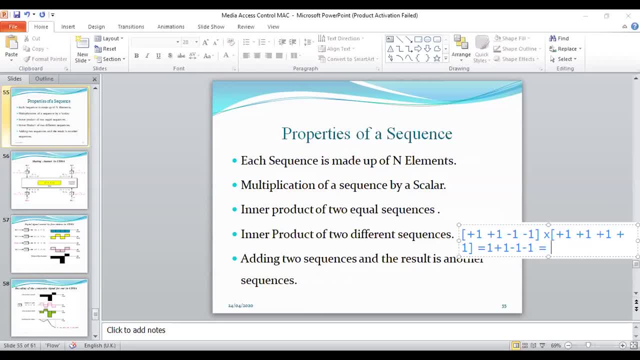 it here is supposed to be minus one. it here is supposed to be minus one, right? what is the end result? you are right. what is the end result? you are right. what is the end result? you are going to get it going to get it going to get it. what is the end result supposed to be? and? 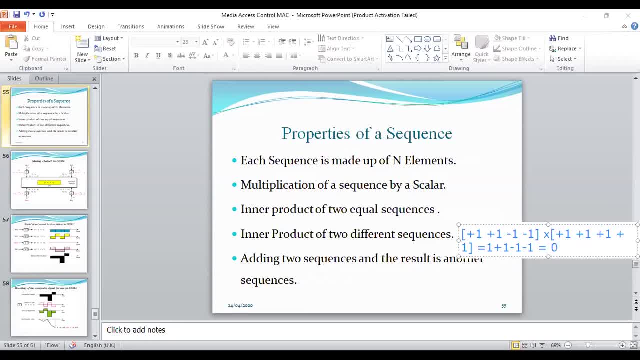 what is the end result supposed to be and what is the end result supposed to be, and these are supposed to be, what these are supposed to be, what these are supposed to be, what here is zero end result is supposed to be. here is zero end result is supposed to be. 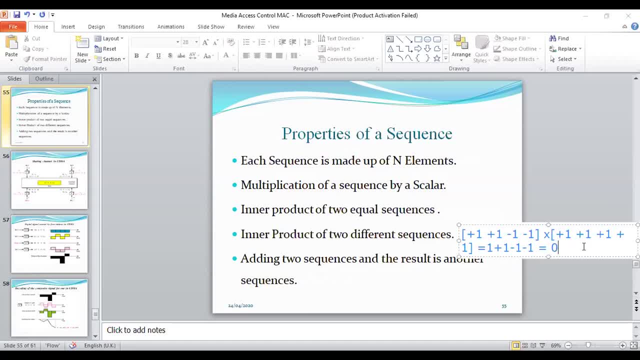 here is zero. end result is supposed to be and result is supposed to be zero. here and result is supposed to be zero here and result is supposed to be zero here. right and result is supposed to be zero. right and result is supposed to be zero. right and result is supposed to be zero. inner product of two different sequences. 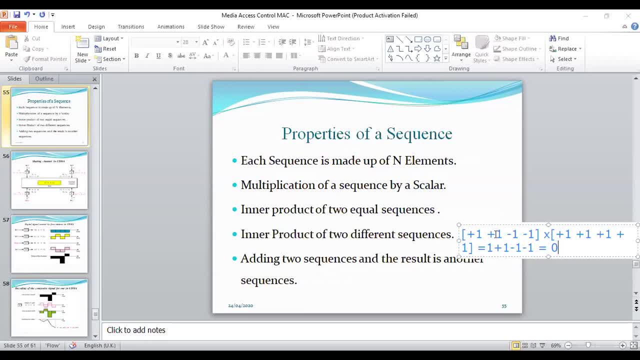 inner product of two different sequences. inner product of two different sequences. this is the first sequence. this is the first sequence. this is the first sequence. you have a different element. this is plus. you have a different element. this is plus. you have a different element: this is plus one. plus one. minus one. minus one. 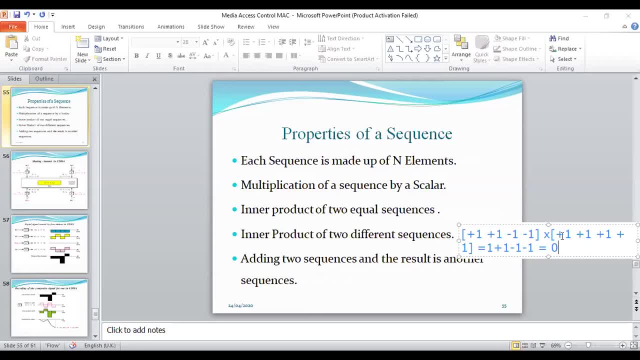 one plus one minus one, minus one. one plus one minus one minus one. second sequence is having, is having. a second sequence is having, is having. a second sequence is having. a different elements: here all are plus one. different elements: here all are plus one. different elements: here all are plus one plus one, plus one and plus one. 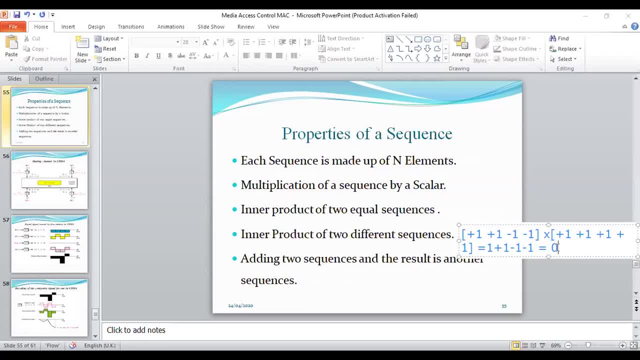 plus one plus one and plus one plus one plus one and plus one. multiply by these two. whatever the multiply by these two, whatever the multiply by these two, whatever the result you are going to get, it is what result you are going to get. it is what result you are going to get. it is what zero. whatever the result you are going. 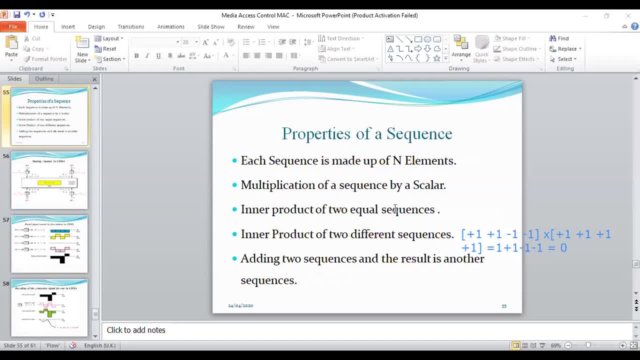 zero. whatever the result you are going: zero. whatever the result you are going to get, it is zero. this case, what happens to get? it is zero. this case, what happens to get, it is zero. this case, what happens? inner product of two equal sequences. inner product of two equal sequences. 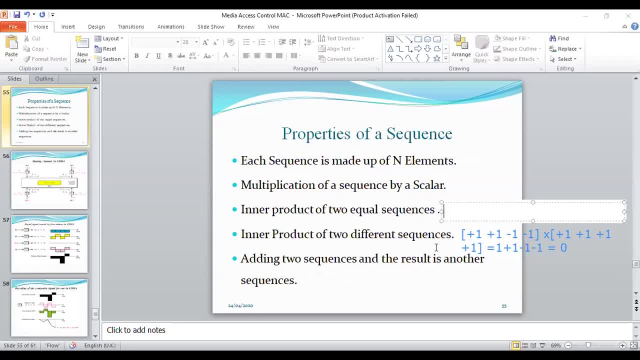 inner product of two equal sequences. the result is supposed to be four. result: the result is supposed to be four. result: the result is supposed to be four. result is supposed to be four. here is supposed to be four. here is supposed to be four here. last one adding two sequences and the. 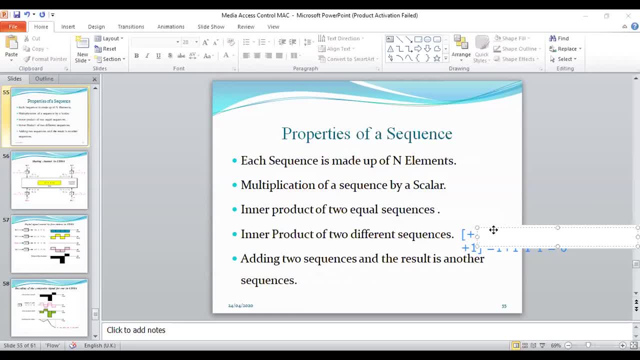 last one adding two sequences and the last one adding two sequences and the result is another sequence. result is another sequence. result is another sequence. right, adding the two sequence and result: right, adding the two sequence and result: right, adding the two sequence and result is: is is another sequence. okay, result is another. 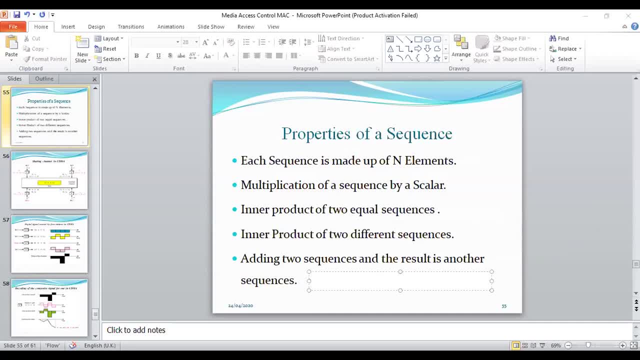 another sequence, okay, result is another. another sequence, okay. result is another sequence. we'll take sequence, we'll take sequence, we'll take. what is this? adding the this one here, you. what is this adding the this one here, you? what is this adding the this one here? you can see adding two sequences. 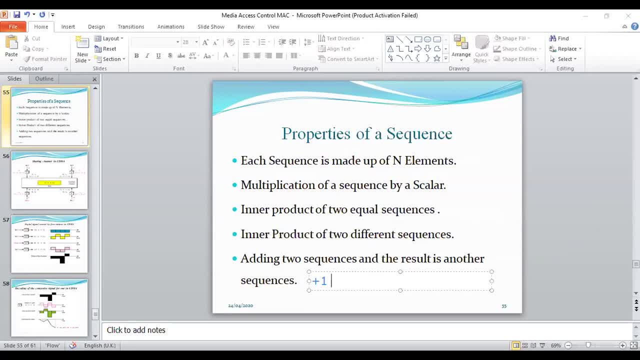 can see adding two sequences. can see adding two sequences. you can add two sequence, for example: plus. you can add two sequence, for example: plus. you can add two sequence, for example: plus one, one, one and plus one then and plus one then and plus one, then sequence also. you take any, uh. second: 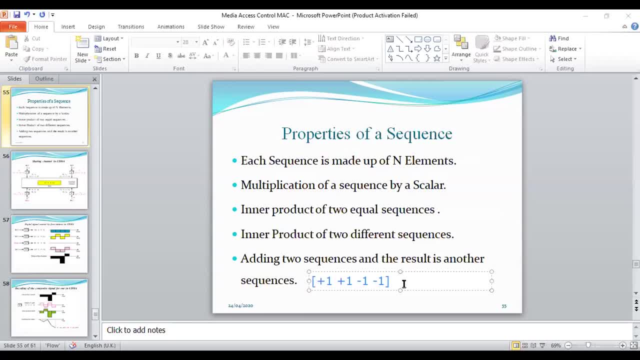 sequence also. you take any uh. second sequence also. you take any uh second sequence, you need to add it. add two sequence, you need to add it. add two sequence, you need to add it. add two sequences here plus sequences here, plus sequences here, plus right, what is supposed to? you need to. 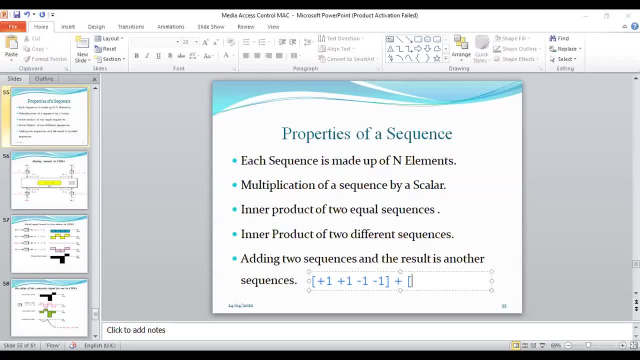 what is supposed to. you need to. what is supposed to, you need to. add it plus right. add it plus right, add it plus right. then you take another sequence, for then you take another sequence, for then you take another sequence, for example, plus one example, plus one example, plus one right. you take one more sequence as plus. 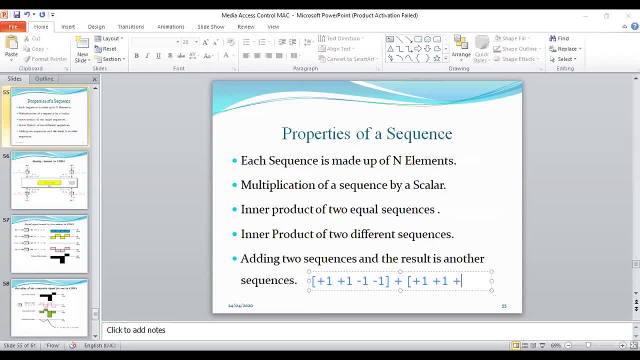 right, you take one more sequence as plus. right, you take one more sequence as plus one. you take one more sequence as one. you take one more sequence as one. you take one more sequence as maybe a plus one, maybe a plus one, maybe a plus one. right, you take one more sequence as plus. 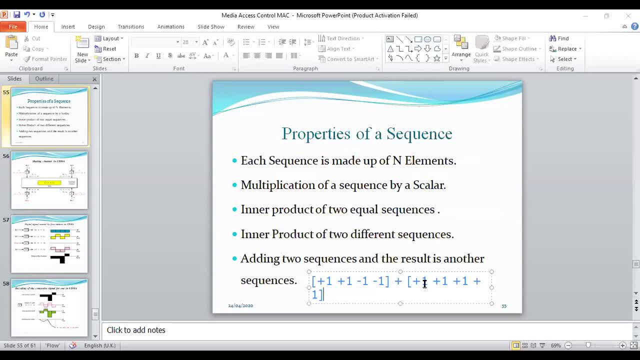 right, you take one more sequence as plus. right, you take one more sequence as plus one, one, one. you take one more sequences plus one. now you take one more sequences plus one. now you take one more sequences plus one. now you add these two. what is the value? 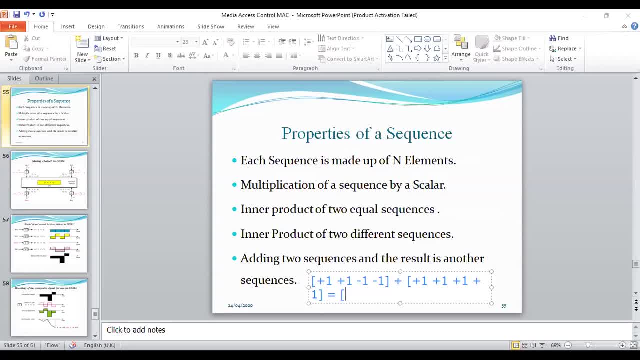 you add these two. what is the value? you add these two. what is the value? you're going to get it here. you're going to get it here. you're going to get it here, the resultant sequence, what you're the resultant sequence, what you're the resultant sequence, what you're supposed to get it here is: 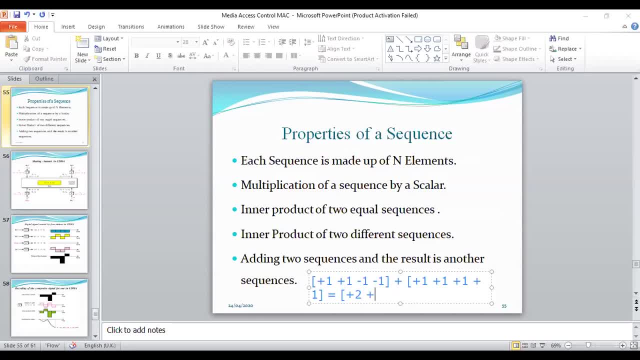 supposed to get it. here is supposed to get it. here is plus two, then you'll get again plus two plus two. then you'll get again plus two plus two. then you'll get again plus two. right this and this you need to add it. right, this and this you need to add it. 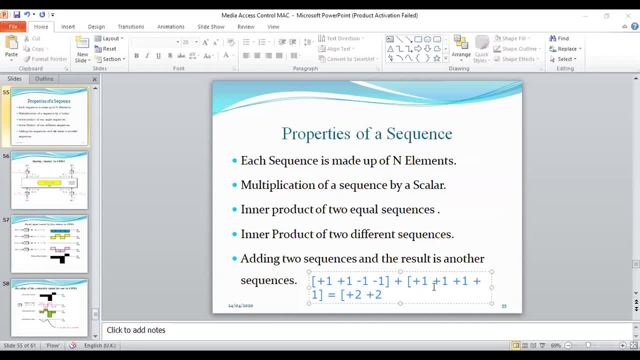 right, this and this. you need to add it: how much you get it plus two now the? how much you get it plus two now, the. how much you get it plus two now the second element plus two. second element plus two. second element plus two. answer: plus one and plus one plus one. 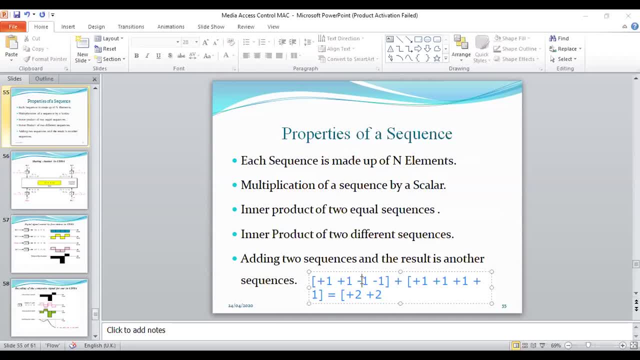 answer: plus one and plus one, plus one. answer: plus one and plus one. plus one and plus one: you add, it is become plus. and plus one: you add, it is become plus. and plus one: you add, it is become plus two. the third element is: what minus one? two. the third element is what minus one two. the third element is what minus one and the plus one. what is the result? you and the plus one? what is the result you and the plus one? what is the result you are going to get it? the result is: 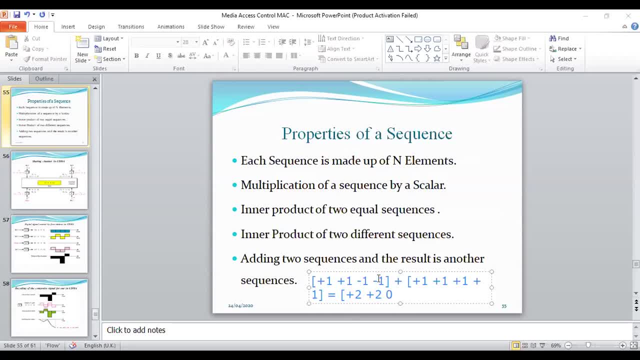 are going to get it. the result is: are going to get it. the result is supposed to be zero. supposed to be zero. supposed to be zero then. what is the fourth element? fourth then? what is the fourth element? fourth then? what is the fourth element fourth element is minus one and minus one, and 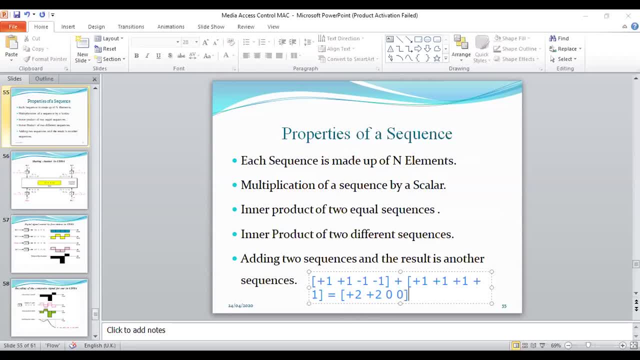 element is minus one and minus one, and element is minus one and minus one and the plus one. what is the result? is zero the plus one. what is the result? is zero the plus one. what is the result is zero, right, right, right. result is zero. this is the uh last. 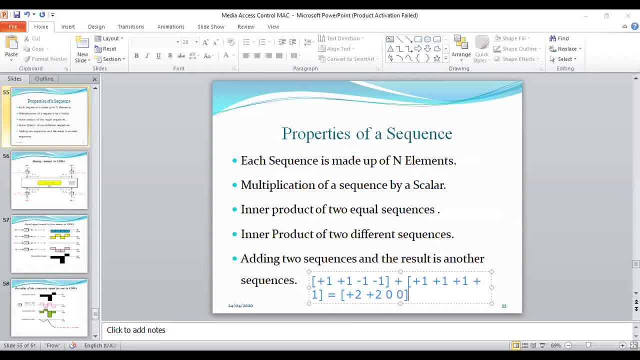 result is zero. this is the uh last result is zero. this is the uh last. property of a sequence: adding. property of a sequence: adding property of a sequence, adding, adding two sequences, and the result is adding two sequences, and the result is adding two sequences, and the result is a result is another sequence now, whatever. 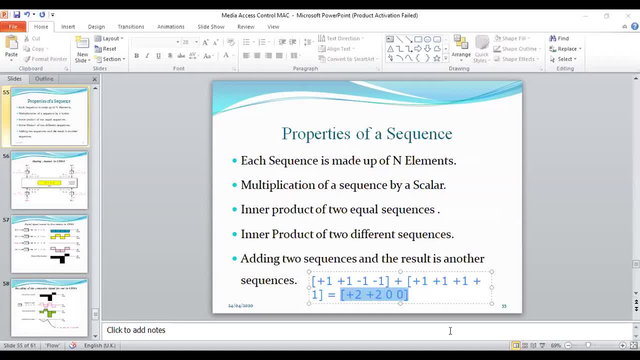 a result is another sequence now. whatever a result is another sequence now. whatever the sequence you got, it is another. the sequence you got, it is another. the sequence you got, it is another, sequence totally different. sequence here. sequence totally different. sequence here. sequence totally different, sequence here. you can see this. 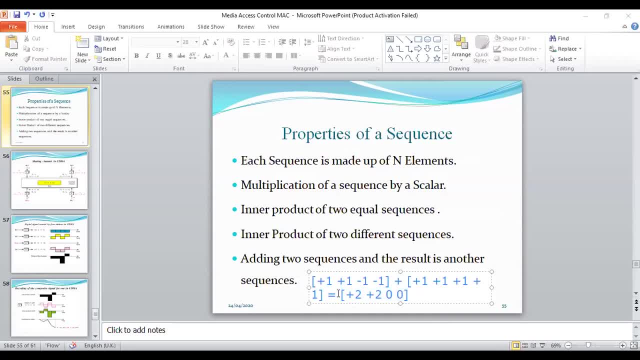 you can see this. you can see this. this is the first sequence. this is the. this is the first sequence. this is the. this is the first sequence. this is the second sequence. you have just added second sequence. you have just added second sequence. you have just added now the. what is the result? you are going. 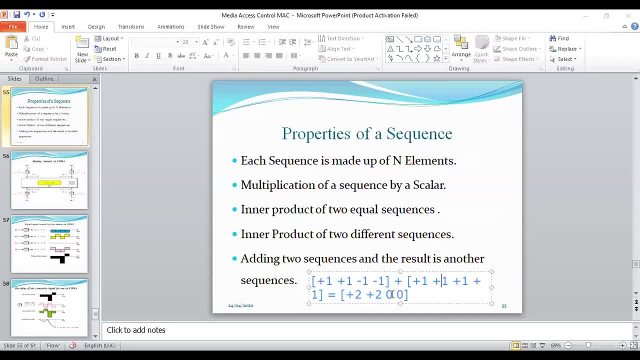 now the. what is the result? you are going now the. what is the result? you are going to get into the third sequence, to get into the third sequence. to get into the third sequence the meaning of zero in the sense that, the meaning of zero in the sense that. 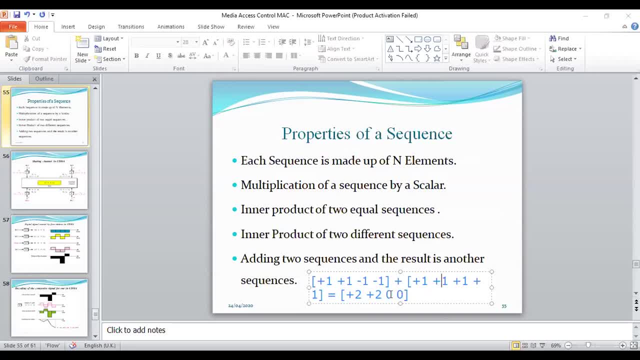 the meaning of zero in the sense that means the particular station is not, means the particular station is not, means the particular station is not sending any data right. the value is sending any data right. the value is sending any data right. the value is supposed to be zero here. 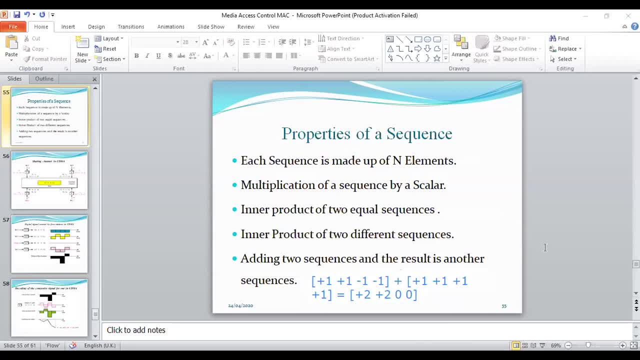 supposed to be zero here? supposed to be zero here? right, this is. these are the properties of right. this is. these are the properties of right this is. these are the properties of a sequence, a sequence, a sequence. okay, these are the properties of a. okay, these are the properties of a. 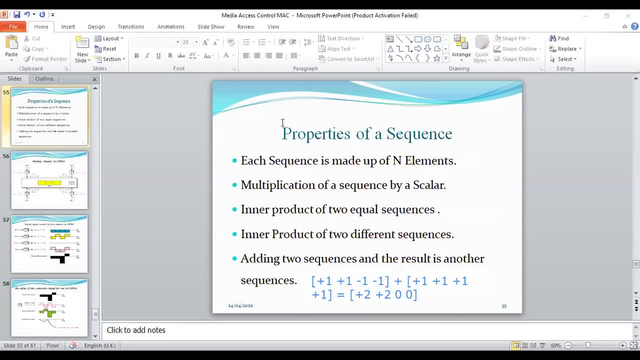 okay, these are the properties of a sequence now, let me come back. sequence now, let me come back. sequence now, let me come back. let me come back to the uh. let me come back to the uh. let me come back to the uh- other topic here- let me come back to. 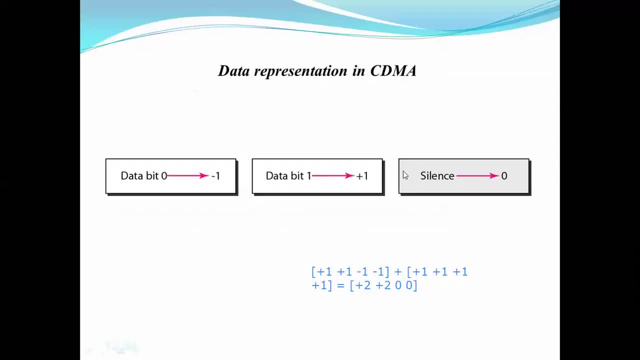 other topic here. let me come back to other topic here. let me come back to the other topic, the other topic, the other topic. come back to the topic data. come back to the topic data. come back to the topic data. representation in cdma. representation in cdma. 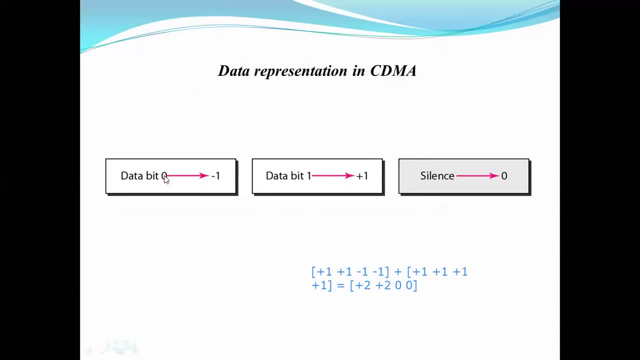 see, as i told you uh earlier right data. see, as i told you uh earlier right data. see, as i told you uh earlier right data bit zero, bit, zero, bit zero. suppose the particular station is. suppose the particular station is. suppose the particular station is sending the data to zero. 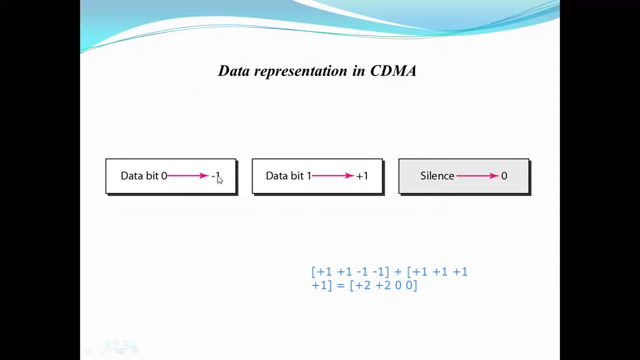 sending the data to zero. sending the data to zero. that means the data element you are. that means the data element you are. that means the data element you are going to represent with the sequence is going to represent with the sequence is going to represent: with the sequence is minus one. 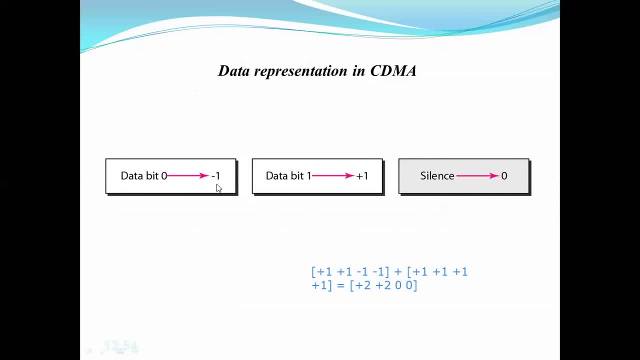 minus one, minus one in the sequence you have to represent in the sequence you have to represent in the sequence you have to represent the data element right, the element you, the data element right, the element you, the data element right, the element you need to represent, need to represent. 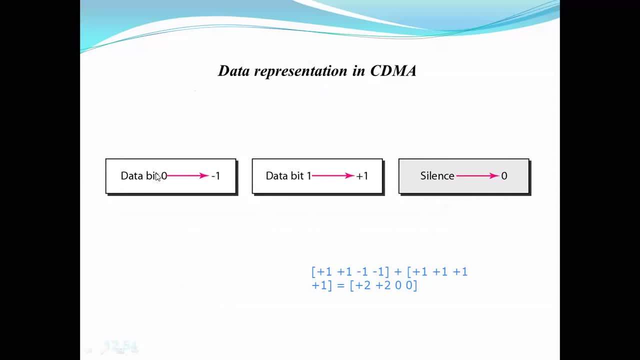 need to represent whenever it comes to, whenever it, whenever it comes to whenever it, whenever it comes to whenever it represents as minus one. that means the represents as minus one. that means the represents as minus one. that means the particular station is sending the data. particular station is sending the data. 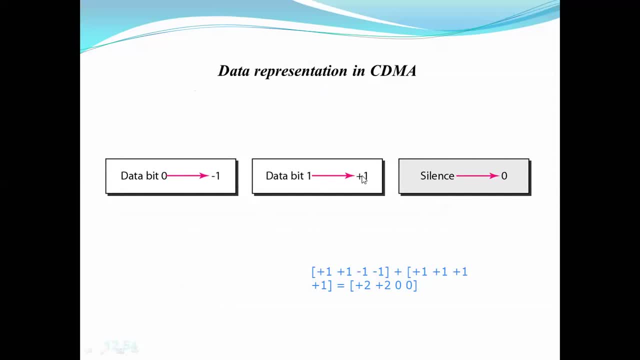 particular station is sending the data as zero data beta is zero. as zero data beta is zero. as zero data beta is zero. whenever you are representing the, whenever you are representing the, whenever you are representing the data element in this sequence element in data element in this sequence element in. 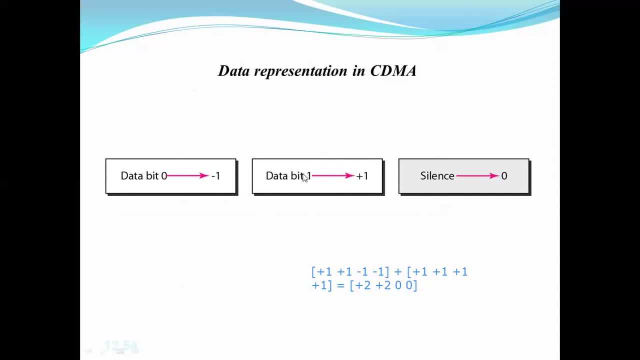 data element in this sequence. element in the sequence as plus one. that means the. the sequence as plus one, that means the. the sequence as plus one. that means the particular station is sending the data. particular station is sending the data. particular station is sending the data, bit as: 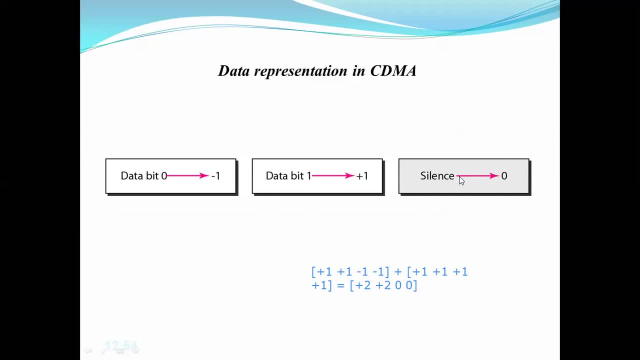 bit as bit as one. suppose the particular station is one. suppose the particular station is one. suppose the particular station is silent. if the particular station is silent, if the particular station is silent, if the particular station is silent, then uh, what is the meaning here? silent then, uh, what is the meaning here? 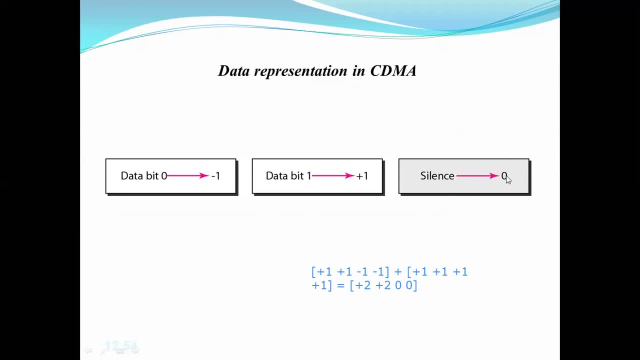 silent then. uh, what is the meaning here? uh, you need to. you are representing the. uh, you need to. you are representing the uh, you need to. you are representing the element in a sequence as zero. you are element in a sequence as zero. you are element in a sequence as zero. you are representing the element as zero here. 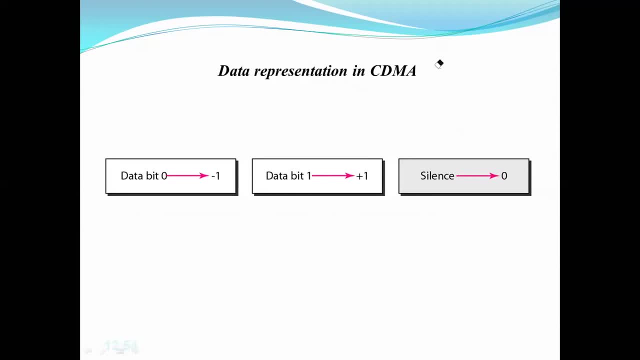 representing the element as zero here. representing the element as zero here. zero here, okay, zero here. okay, zero here. okay, that's zero here. that's zero here. that's zero here. so uh, this is how uh the data. so uh, this is how uh the data. so uh, this is how uh the data. representation normally happens in the. 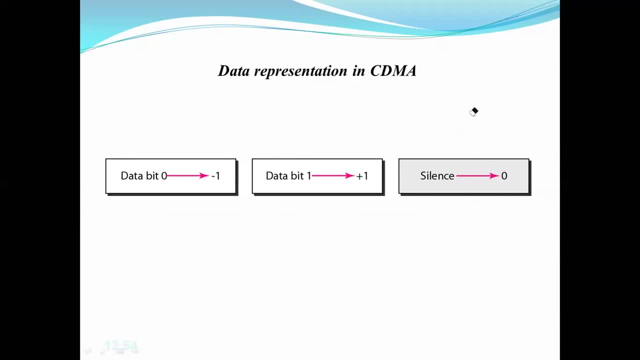 representation normally happens in the representation normally happens in the cdma right cdma now. let me move on to another cdma now. let me move on to another cdma now. let me move on to another. important one is uh sharing the channel. important one is uh sharing the channel. 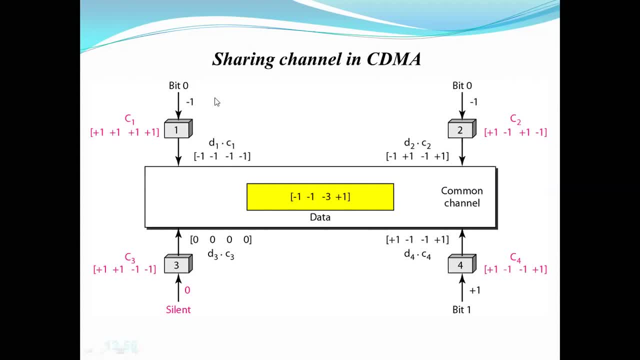 important one is uh sharing the channel in cdma, in cdma, in cdma. what happens, uh, there are four stations. what happens, uh, there are four stations. what happens, uh, there are four stations. you can see here, you can see here, you can see here, uh, there are four stations, you can see. 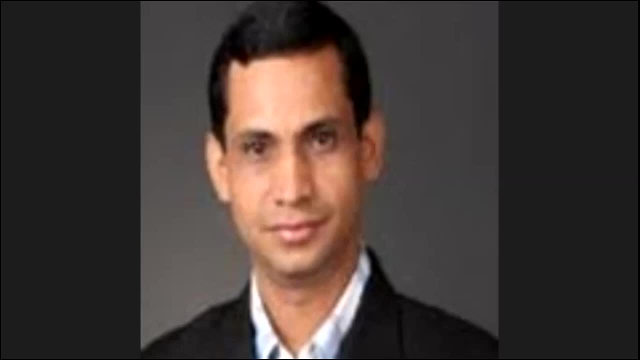 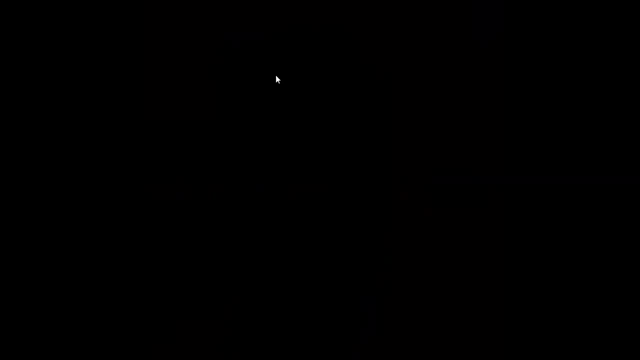 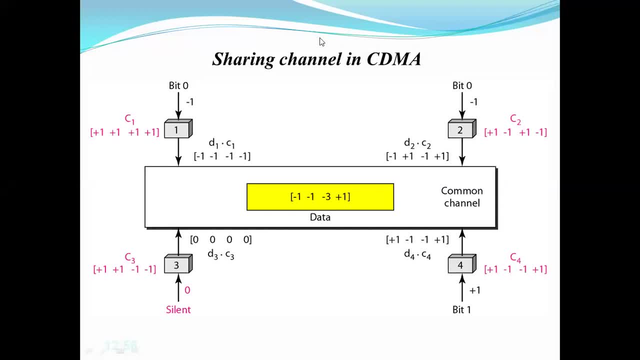 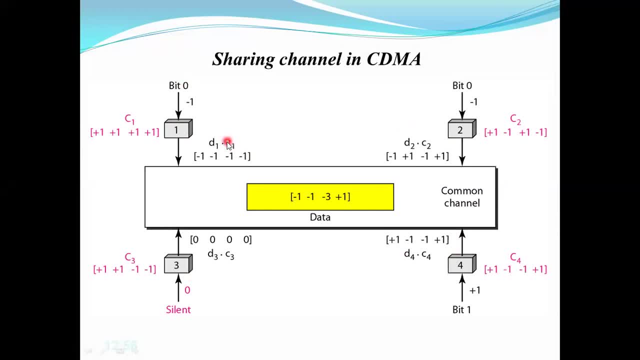 you can see station one, station two. you can see station one, station two, station three and station four: right now. station three and station four right now. station three and station four right now. uh d1 is the data of the station one and uh d1 is the data of the station one and. 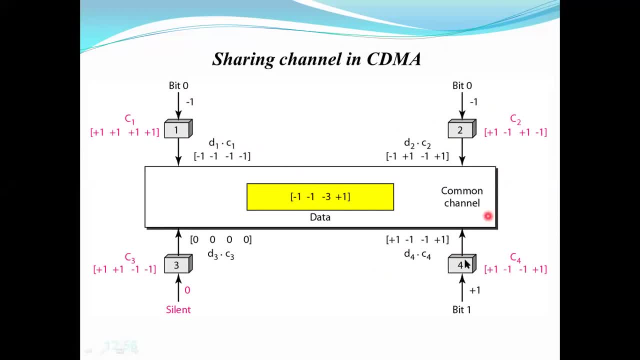 uh, d1 is the data of the station one and c1 is the c1 is the c1 is the code of the station one like this: it code of the station. one like this: it code of the station. one like this: it applies to all other stations. 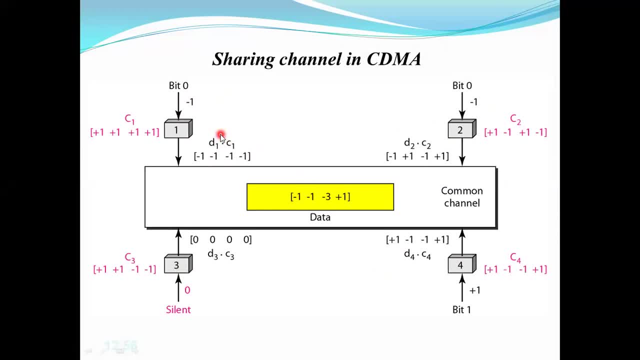 applies to all other stations. applies to all other stations. right now. when it multiplies d1 and c1. right now, when it multiplies d1 and c1, right now, when it multiplies d1 and c1, the c1 is for the station, one is plus one. 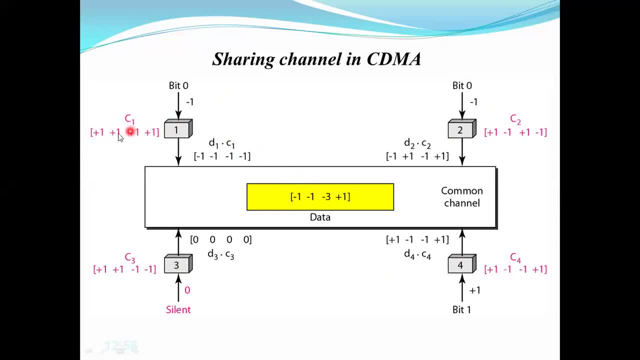 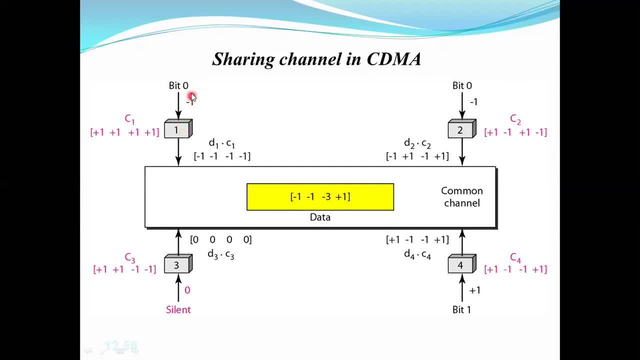 code sequence: the sequence of the code sequence. the sequence of the station: one right station. sequence of the station one right station. sequence of the station one right station. sequence of the station mark, station mark, station mark and whatever the bit it suppose you are and whatever the bit it suppose you are. 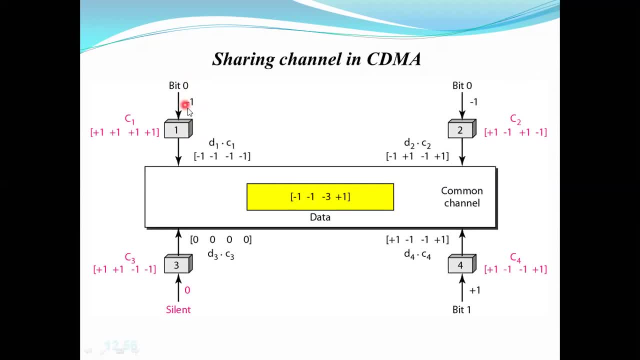 and whatever the bit it suppose you are sending is zero. that means sending is zero. that means sending is zero. that means minus one. right minus one. right minus one. minus one. right minus one. minus one, right minus one. you need to multiply with this, multiply. you need to multiply with this multiply. 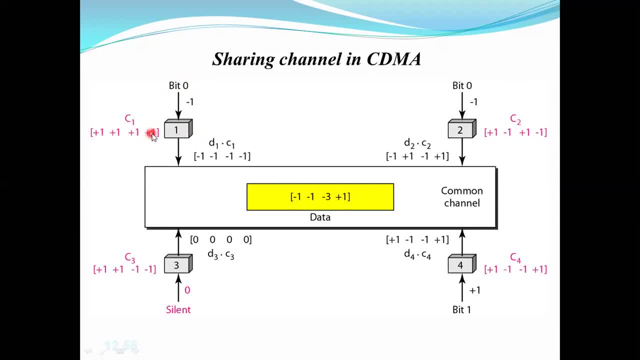 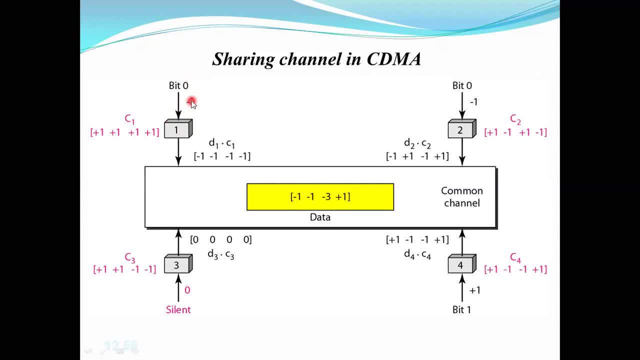 plus one. this is what the sequence plus one. this is what the sequence, this sequence multiplied with the data data, this sequence multiplied with the data data. this sequence multiplied with the data data, is what minus one here multiply with. is what minus one here multiply with. is what minus one here multiply with that. what is actually the resultant is. 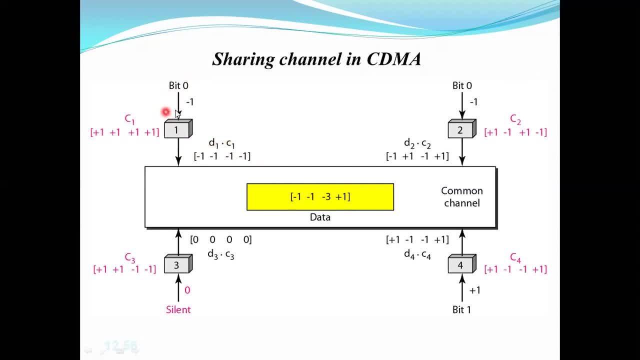 that what is actually the resultant is that what is actually the resultant is: d1 multiplied by c1, that means plus one. d1 multiplied by c1, that means plus one. d1 multiplied by c1, that means plus one. multiplied by minus, one is become minus. 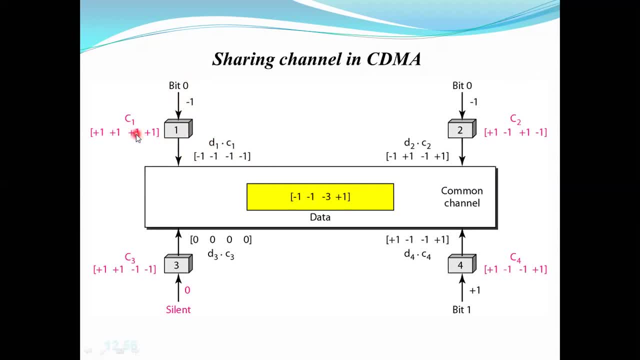 multiplied by minus one is become minus. multiplied by minus one is become minus. one plus one. multiplied minus one is one plus one. multiplied minus one is one plus one. multiplied by minus one is one plus one. multiplied by minus one is minus one. then plus one, minus one, minus. minus one, then plus one minus one minus minus one, then plus one minus one minus one. plus one minus one minus one. this is one plus one minus one minus one. this is one plus one minus one minus one. this is what a result you are going to get it. 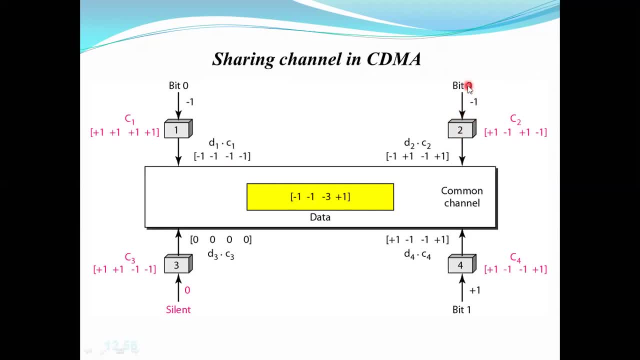 what a result you are going to get it. what a result you are going to get it. similarly, all other stations here also. similarly, all other stations here also. similarly, all other stations here also. bit uh, let us take this station number. bit uh, let us take this station number. 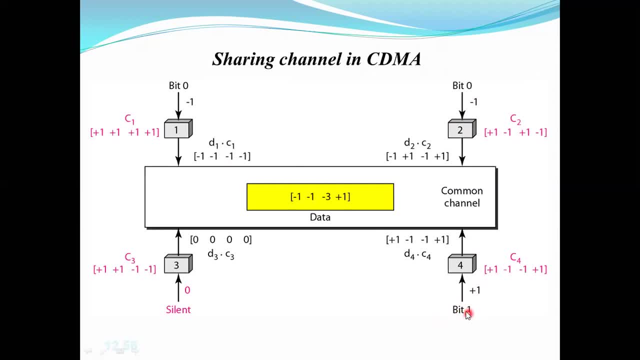 bit. uh, let us take this station number four here. station four is sends the bit four here. station four is sends the bit four here. station four is sends the bit as one as one as one. sends the bit as one, that means the, sends the bit as one, that means the. 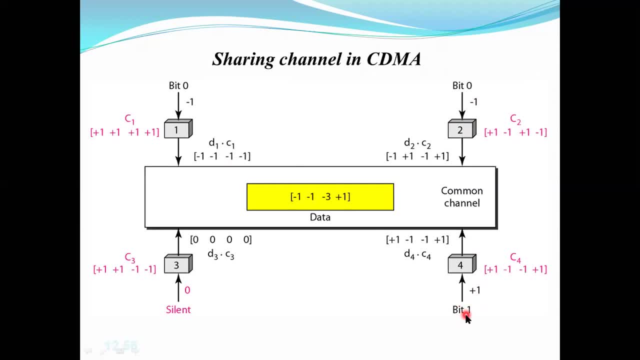 sends the bit as one. that means the element. you are going to represent as element. you are going to represent as element. you are going to represent as plus one. you are representing as plus plus one. you are representing as plus plus one. you are representing as plus one right. 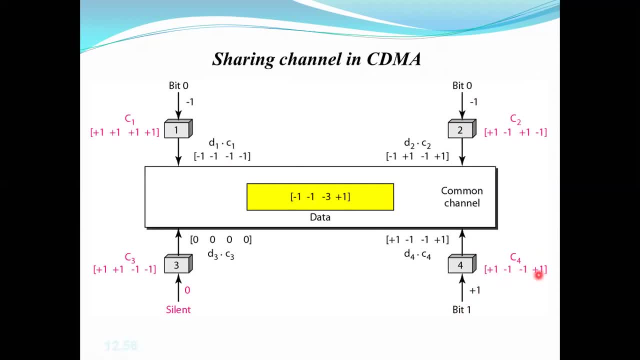 one right, one right. what is the code of the c4 here? the. what is the code of the c4 here, the. what is the code of the c4 here? the station four is plus one minus one. station four is plus one minus one. station four is plus one minus one minus one plus four. 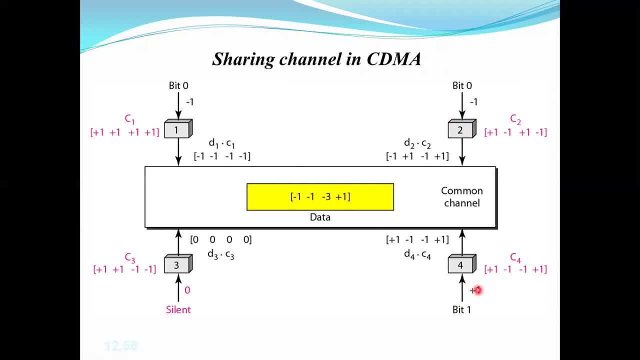 minus one plus four. minus one plus four. now this data, now this data, now this data. you need to multiply with the code here. you need to multiply with the code here. you need to multiply with the code here: right plus one multiplied by plus one. right plus one multiplied by plus one. right plus one multiplied by plus one. what is the result? you are going to get right plus one multiplied by plus one. what is the result? you are going to get right plus one multiplied by plus one. what is the result? you are going to get it here. it here. 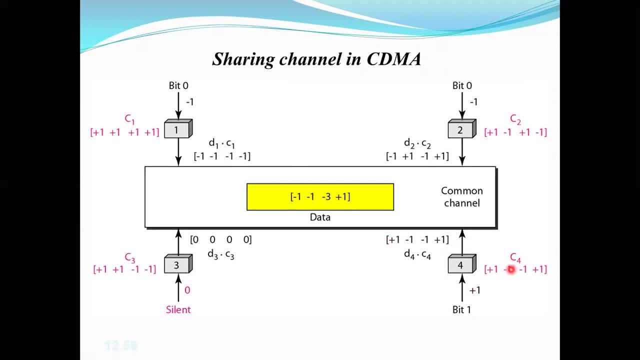 it here plus one. you are going to get it as plus plus one. you are going to get it as plus plus one. you are going to get it as plus one. now, plus one is multiplied with one. now, plus one is multiplied with one. now, plus one is multiplied with minus one. what is the result? you are 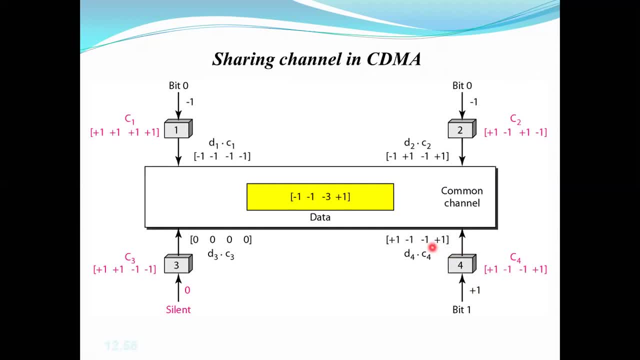 minus one. what is the result? you are minus one. what is the result you are going to get? is a minus one now plus one going to get. is a minus one now plus one going to get. is a minus one now plus one, multiplied by minus one. you are going to. 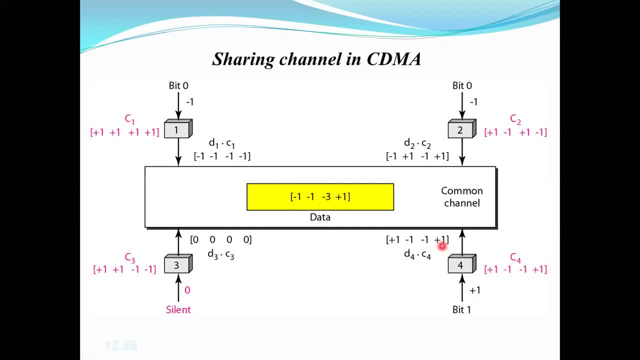 multiplied by minus one, you are going to. multiplied by minus one, you are going to get a minus one plus one is multiplied. get a minus one plus one is multiplied. get a minus one is multiplied with the plus one. what is the result? you with the plus one. what is the result? you? 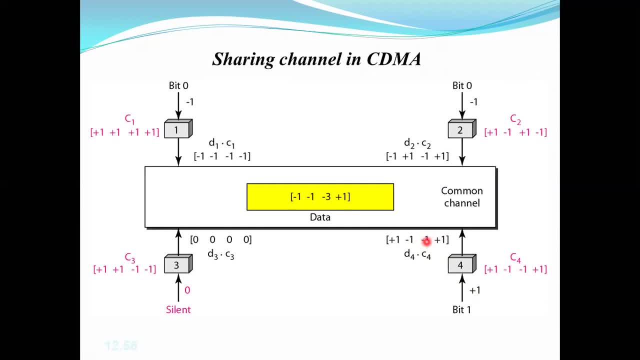 with the plus one. what is the result? you are going to get it is a plus one. are going to get it is a plus one. are going to get it is a plus one. this is what you are going to get it get. this is what you are going to get it get. 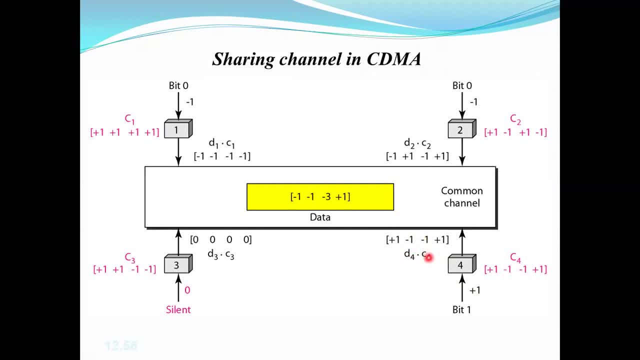 this is what you are going to get it. get it as d4 multiplied by c4. it as d4 multiplied by c4. it as d4 multiplied by c4. right, and this is how you can represent right. and this is how you can represent right and this is how you can represent. imagine, in this case, what happens: station. 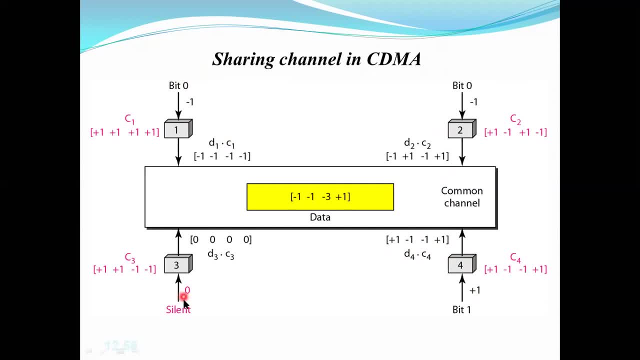 imagine, in this case, what happens station. imagine in this case, what happens station one, station two and station three. one station two and station three one. station two and station three are sending the data here and station are sending the data here and station are sending the data here and station three is a state. you can see the station. 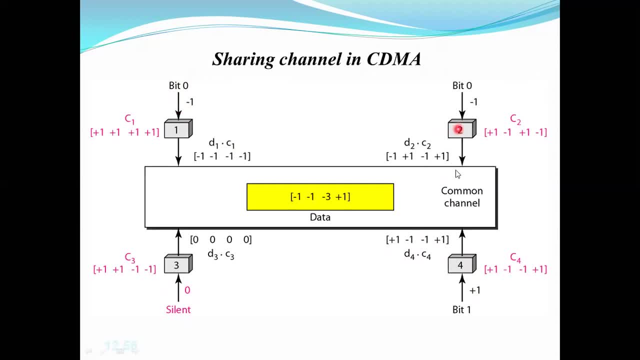 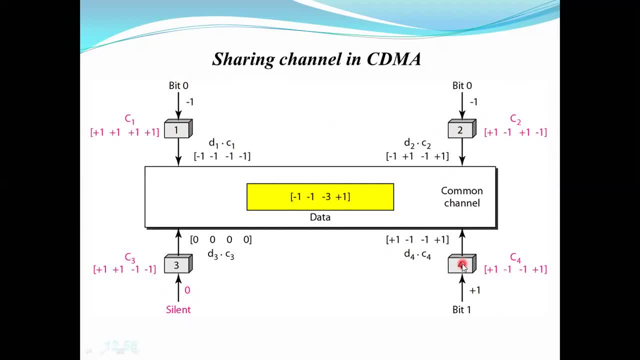 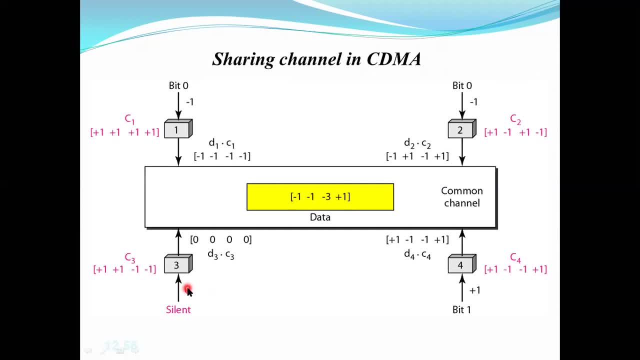 but station three is silent, silent means. but station three is silent. silent means what? how do you represent as zero? what, how do you represent as zero? what, how do you represent as zero, right as zero? now, imagine now station right as zero now. imagine now station right as zero. now, imagine now station three wants to hear from station two. 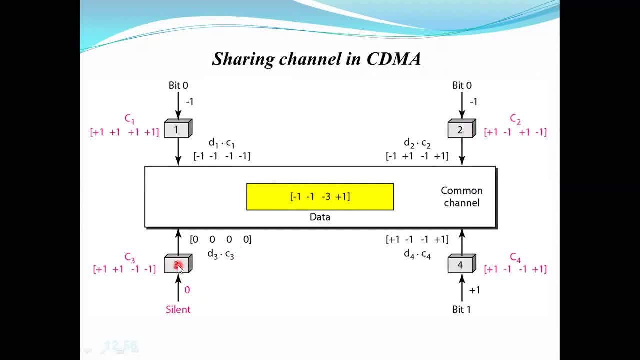 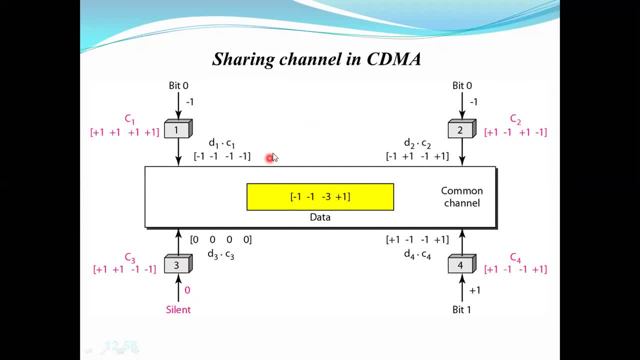 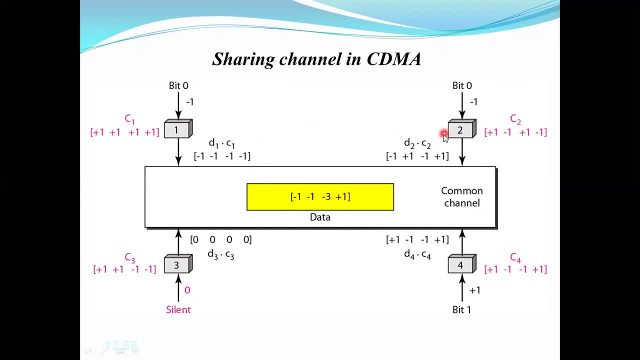 see the summation of all the data. what see the summation of all the data? what you're going to send? you're going to send. you're going to send: uh, along with this channel, the summation. uh, along with this channel, the summation, uh, along with this channel, the summation you need to find out, the summation of. you need to find out the summation of. you need to find out the summation of: sum of all the data. what you're going to sum of all the data. what you're going to sum of all the data. what you're going to send along with. 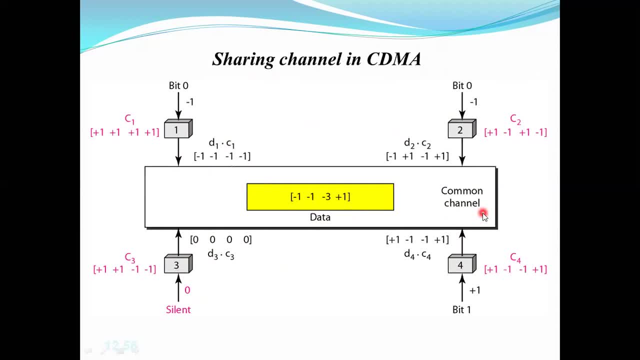 send along with. send along with the in a single channel, right, you need the in a single channel, right. you need the in a single channel, right. you need to take that you have to multiply with. to take that you have to multiply with. to take that you have to multiply with, you have to multiply with the code of. 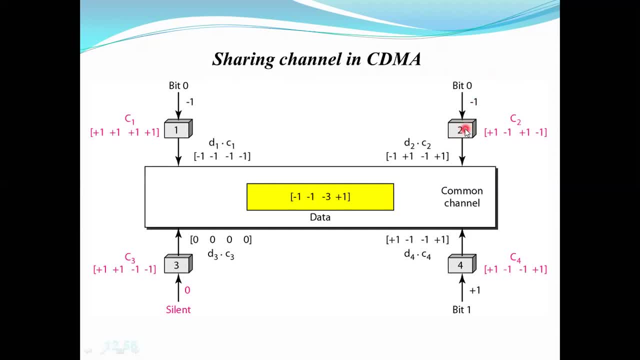 you have to multiply with the code of. you have to multiply with the code of the the the station two. you need to multiply with station two. you need to multiply with station two. you need to multiply with the code of the station two. what is the? the code of the station two? what is the? the code of the station two. what is the code of the station two? what is the the code of the station two. what is the code of the station two here. code of the station two here. code of the station two here. plus one minus one. plus one minus one. 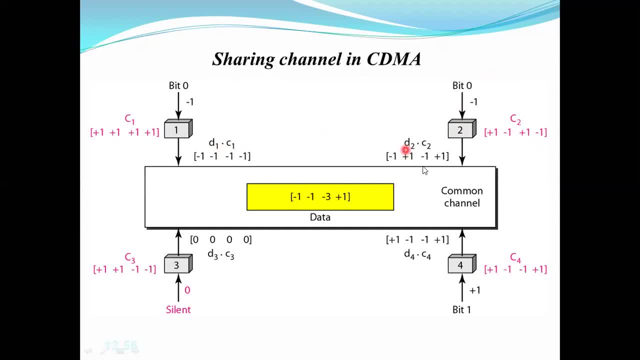 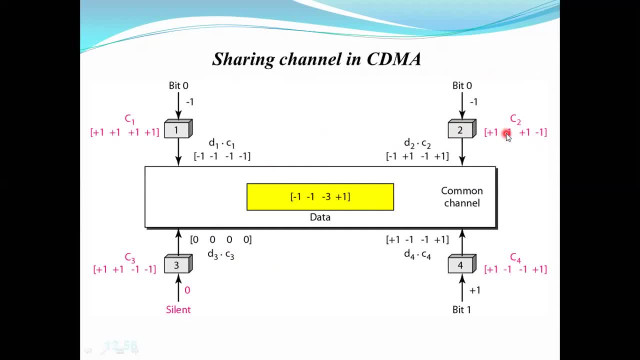 right. the sum of all the data is you right? the sum of all the data is you need to take it and you need to multiply. need to take it and you need to multiply, need to take it and you need to multiply this, this, this, uh. code of station two. now, when you 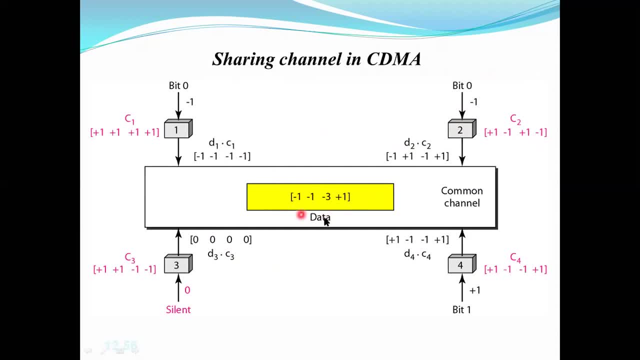 uh code of station two now, when you uh code of station two, now, when you multiply with that, multiply with that, multiply with that, actually the result, what you're going to actually the result, what you're going to actually the result, what you're going to get it is this: 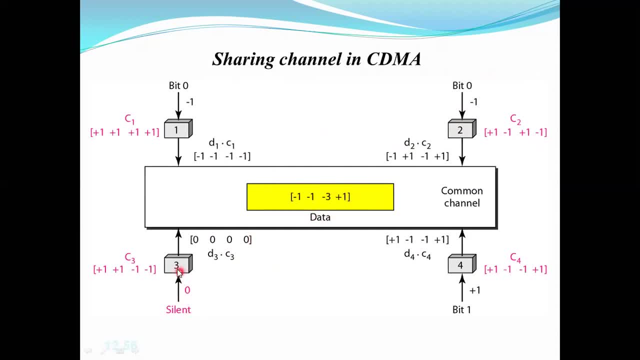 get it is this, get it is this. this is what the result you're supposed to. this is what the result you're supposed to. this is what the result you're supposed to: get it, get it, get it right now they, station three, can able to. right now they, station three, can able to. 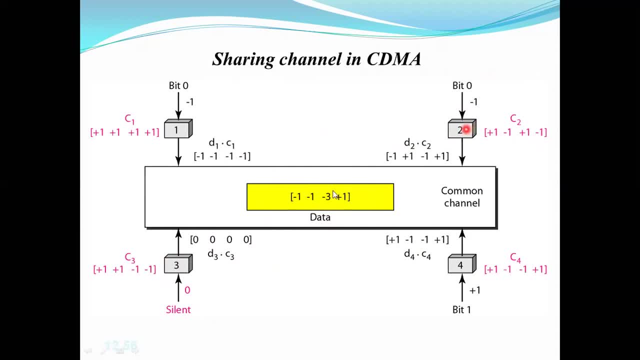 right now they. station three can able to see this particular data. see this particular data. see this particular data. station three can able to hear from station three can able to hear from station three can able to hear from. station two means this particular data. station two means this particular data. 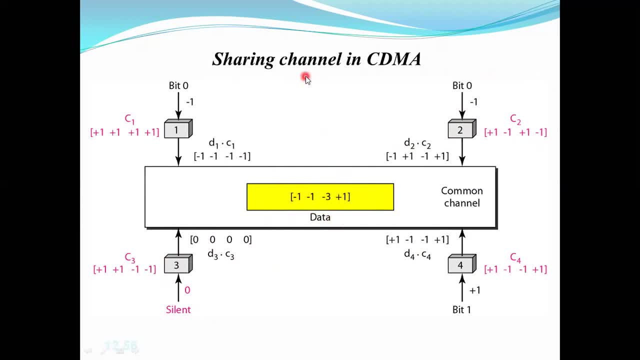 station two means this particular data can able to see it. can able to see it. can able to see it. this is what actually uh uh, you know. this is what actually uh uh, you know. this is what actually uh uh, you know. whenever the station three wants to hear: 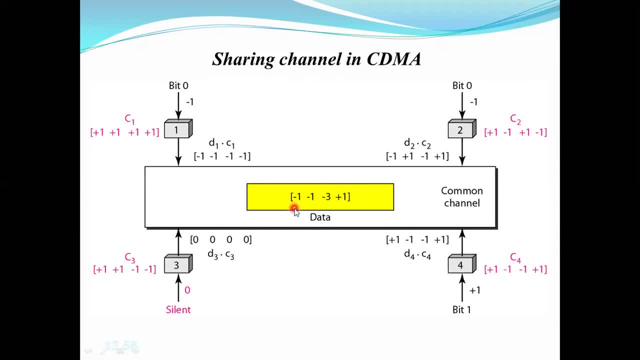 whenever the station three wants to hear, whenever the station three wants to hear from station two. this is how this is how from station two. this is how this is how from station two. this is how this is how you can interpret the interpretation. you can interpret the interpretation. 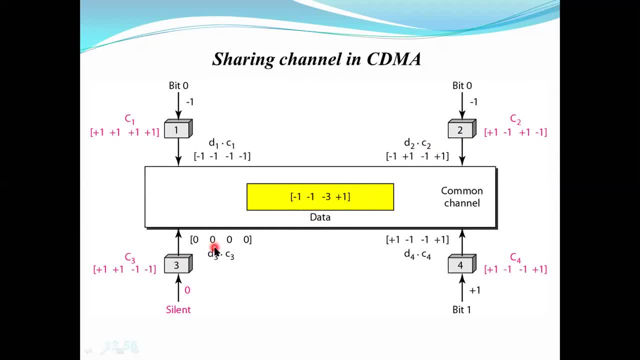 you can interpret. the interpretation happens like this, happens like this, happens like this. interpretation happens like this. okay, interpretation happens like this. okay, interpretation happens like this: okay, now uh, another uh. you can see uh. now uh, another uh. you can see uh. now uh, another uh, you can see uh. the digital signals: 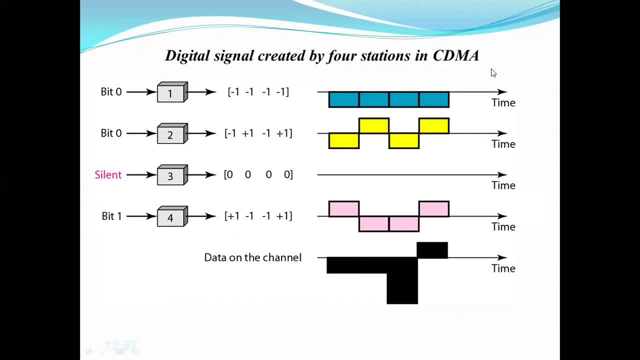 the digital signals. the digital signals right. the signal level will call it as right. the signal level will call it as right. the signal level will call it as. to understand the process easily: the. to understand the process easily. the. to understand the process easily. the digital signal produced by each station. 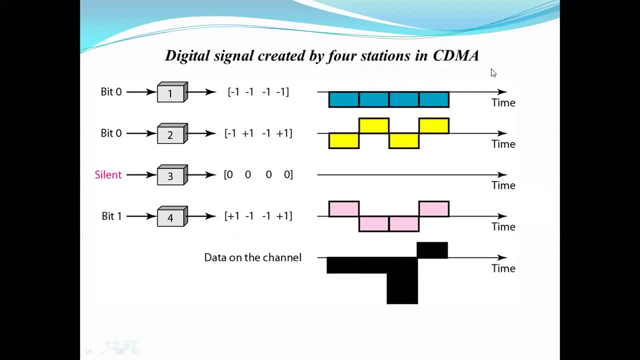 digital signal produced by each station. digital signal produced by each station is represented with the help of a signal, is represented with the help of a signal. is represented with the help of a signal level. now imagine bit zero. okay, the level. now imagine bit zero. okay, the level. now imagine bit zero. okay, the station one is sending the station one. 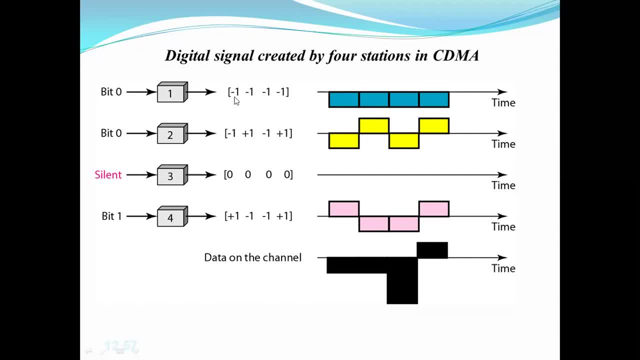 station one is sending the station one. station one is sending the station one. this is what the sequence right sequence, this is what the sequence right sequence, this is what the sequence right sequence bit zero is sending it minus one minus. bit zero is sending it minus one minus. 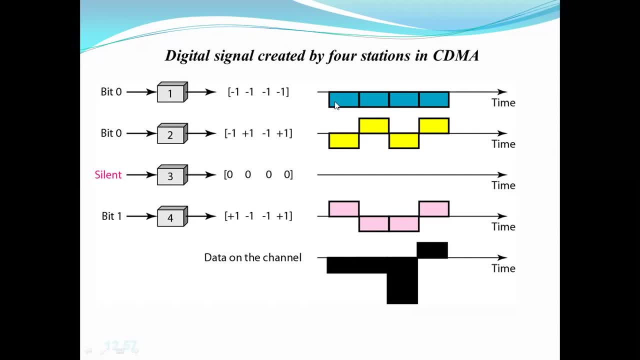 bit zero is sending it minus one minus one minus one. how do you represent? and one minus one? how do you represent? and one minus one? how do you represent? and say, say, say, uh, you know signal level here, because, uh, you know signal level here, because, uh, you know signal level here, because all are minus right. 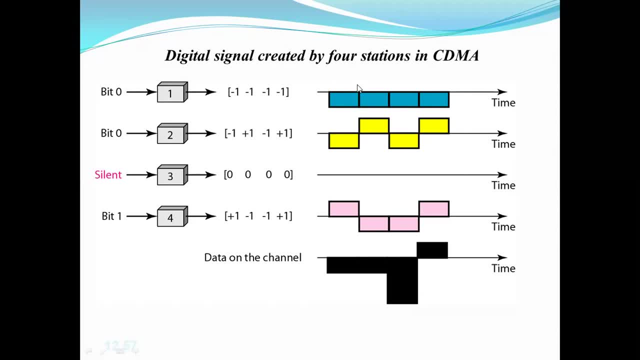 all are minus right, all are minus right below the reference line, below the, below the reference line, below the reference line, below the reference line, reference line, below the reference line. this is what the reference line right, this is what the reference line right, this is what the reference line right, this is what the reference line and. 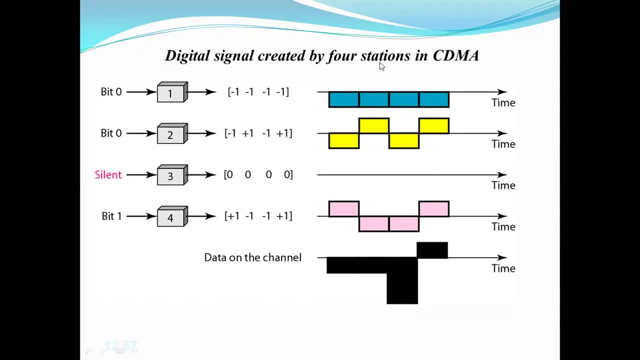 this is what the reference line and this is what the reference line. and below this reference line, you can see, below this reference line, you can see below this reference line, you can see this right, this is the reference. this is what right, this is the reference, this is what. 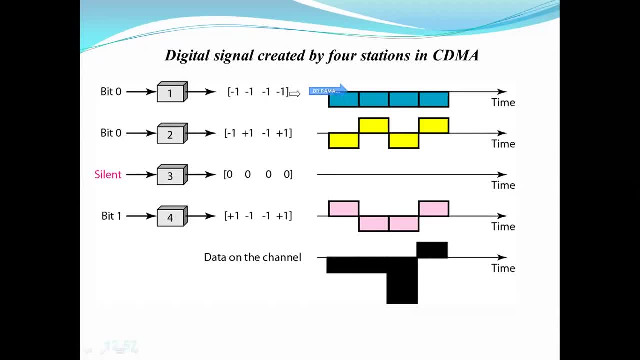 right, this is the reference, this is what the reference line, the reference line, the reference line, but all this minus one, minus one, minus one, but all this minus one, minus one, but all this minus one, minus one, you have it, this is actually. you have it, this is actually. 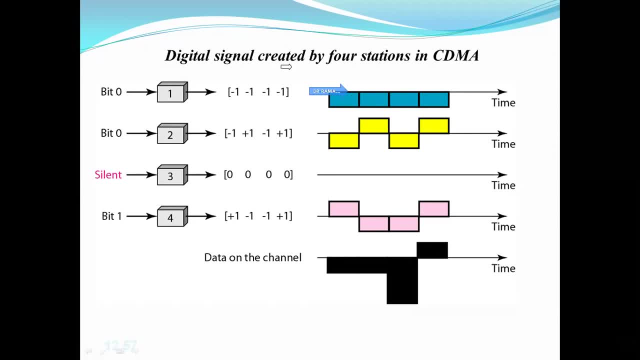 you have it. this is actually below the reference line here, below the below the reference line, here, below the, below the reference line, here below the reference line, right below the reference line. now we imagine the station 2 is sending minus 1 plus 1, minus 1 plus. 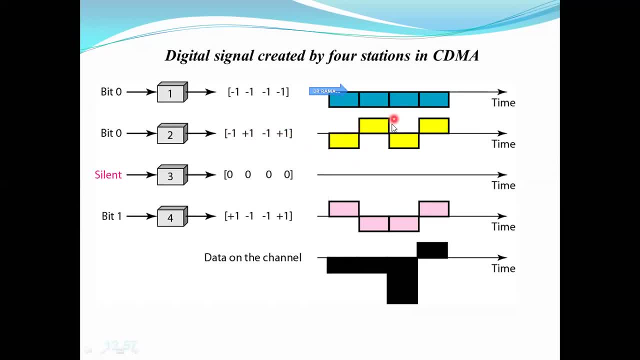 1 initially. what is a minus 1? then it's supposed to be plus 1, right. then again minus 1, then it's going to be plus 1. that is minus plus, minus plus. so easy to understand. right signal level is represented. easy to understand: minus, uh, minus 1 plus 1, minus 1 plus 1.. you take a station 3. 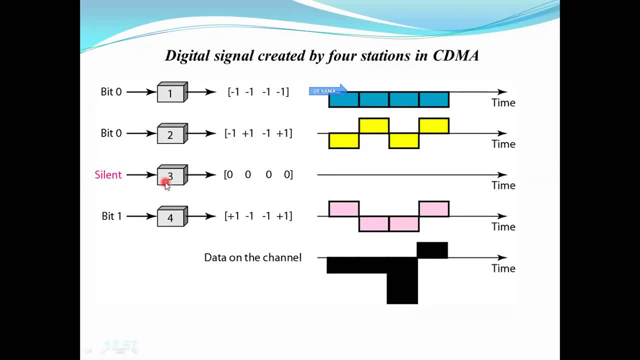 station 3 is what is silent. that means they is not sending any data. that means the value is 0 here. value 0 means what is the straight line? it is a straight line, right, it's a straight line. now let us take the station 4. it's sending the bit 1. that means the sequence is supposed to be what plus 1. 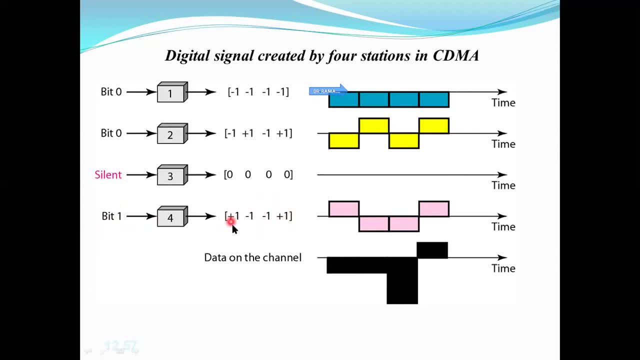 minus 1, minus 1 and the plus 1.. this is what the sequence you were going to get it in the station 4.. now this sequence can be represented with the help of a signal level. that means: the plus 1 plus 1 is what plus 1, this is what the plus 1, then minus 1 minus 1. this is the first minus 1. 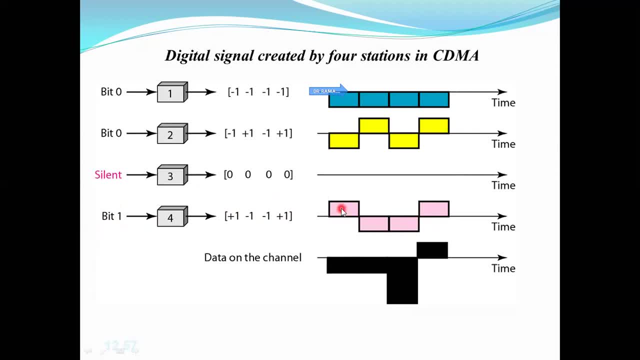 this is the second minus 1 minus 1, minus 1 plus 1 minus 1 minus 1, again plus 1.. this is how you can represent uh the signal levels of the sequence. these sequence can be represented with the help of the signal level, if you see this. 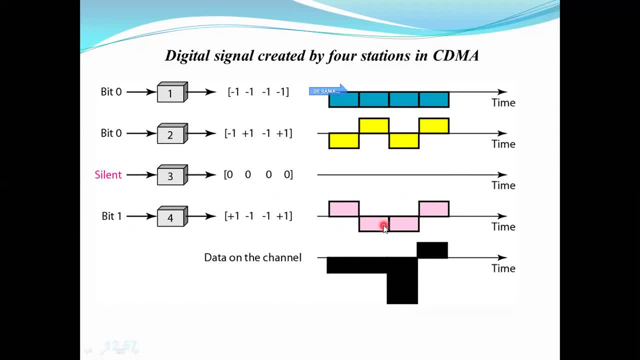 signal level, you can understand easily what is actually a code is right, what is actually a elements in the sequence, what you can understand the sequence very easily with the help of the signal levels. now, data on the channel. data on the channel in the sense, what is actually data? 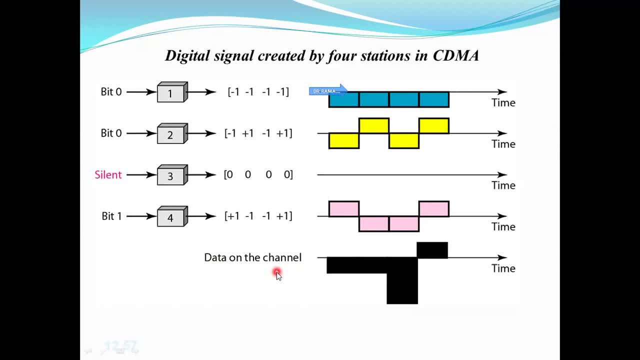 on the channel, some of all the data sent by the station. all the stations are sending the data, right? some of all the datas are sending by the station. that is actually meaning of uh: data on the channel, actual data on the channel that you are representing in this way. right, this is what the data is supposed to. 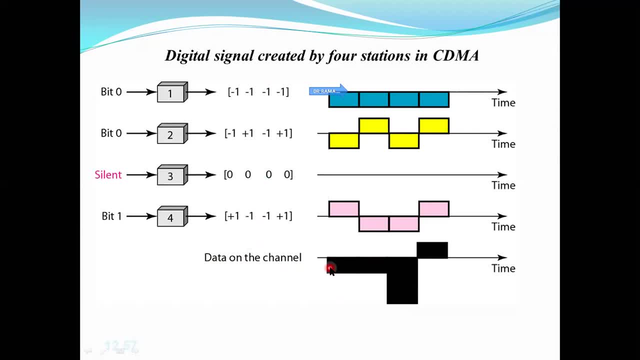 be sending. so if you, you know, add all those things, finally you'll get. this is how you're supposed to get it in the minus. then this minus 3 comes here. you will see, seen here, right the earlier case. there is a uh minus one minus one. then uh minus three. that means plus one, minus one, minus one. 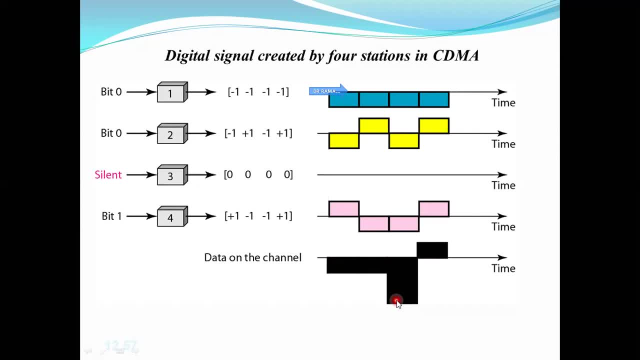 plus minus three, sorry, minus one, minus one, minus three and the plus one. this is what the total data you're going to send it over the channel that we are representing in this uh signal level. this is what the reference line, the below the reference line, above the reference reference time you need. 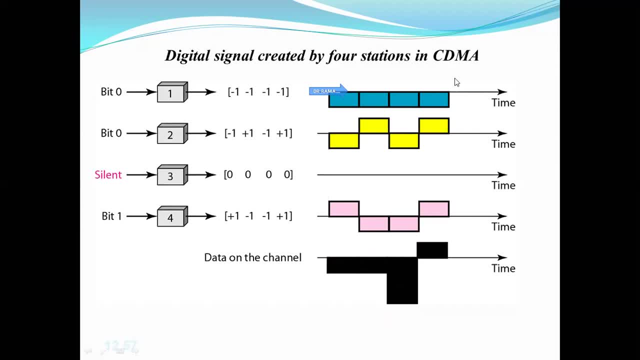 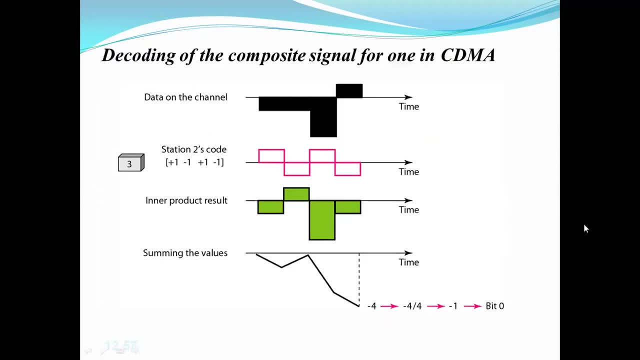 to understand. that is very important, okay, very important here. now, of course it's a. similarly, it applies to the composite signal also. composite signal, in essence, is more than one signal data on the channel. we are represented like this: suppose station three wants to hear, uh, station two, you. 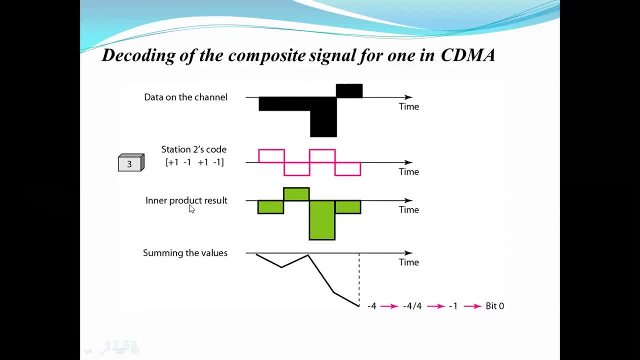 need to multiply with the station code here. this is a station two code, then inner product. if you, if you calculate, okay, whatever the result is the inner product is supposed to get it, then you can represent like this: this is what the inner product is supposed to be. what is that? 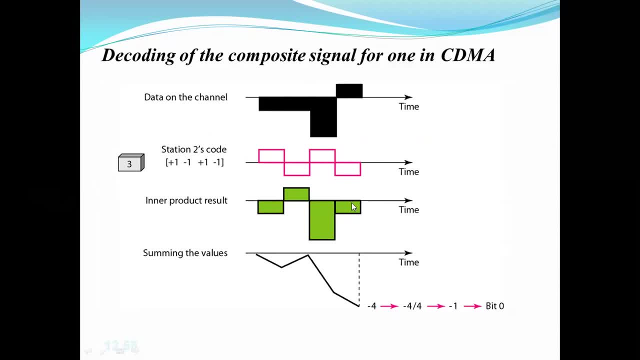 minus one plus one. this is minus three and minus one. then the summing up all the values, what you're supposed to get. it is supposed to be: uh, you're represented as minus four. okay, you need to find out the data. what is the data supposed to be sent? right, that means minus four. 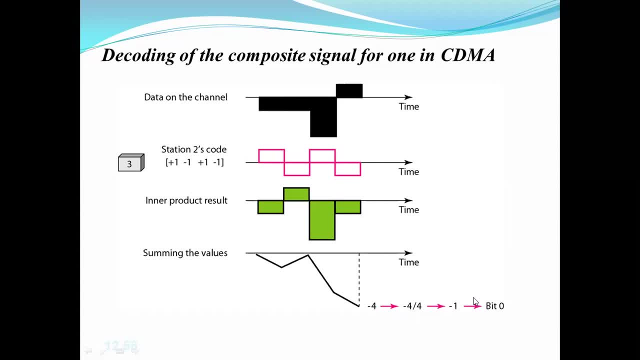 divided by four. that is where you are going to get a data, actual data. the data you're supposed to get it was minus one minus four. divided by four, the result is: what minus one. the meaning of minus one is minus one is supposed to be what zero bit, right? the meaning of minus one is the. 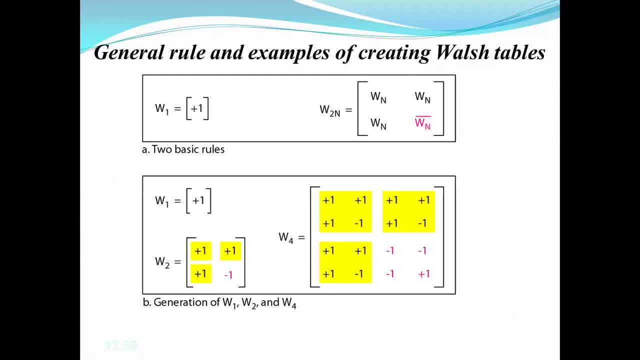 zero bit. that's what the uh meaning here. okay now, uh, the final uh thing which we need to discuss about the walsh tables. okay, about the watch table. now, what is the meaning of walsh table? uh, this is what we normally call it: the signal c to generate a signal. sorry, sequence generation. 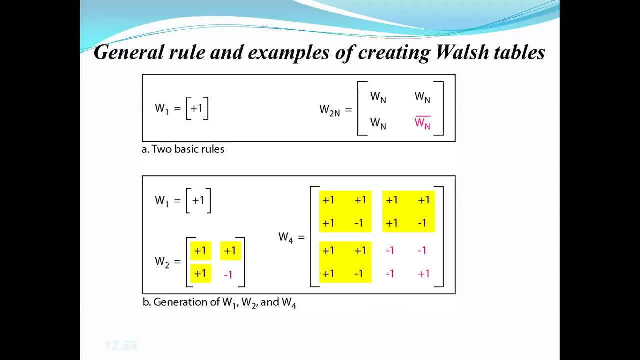 right. you need to generate a sequence right to generate a sequence, normally we'll use the walsh tables to generate a chip sequence. we use a walsh table, which is two-dimensional table, with an equal number of rows as well as columns, to generate a chip sequence. 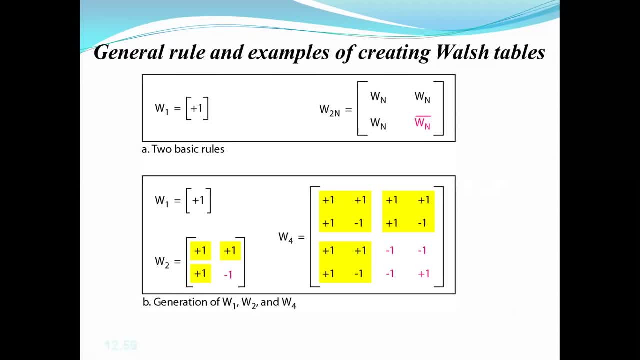 we use a walsh table, which is two-dimensional table, with an equal number of rows as well as columns. now, if we can refer this particular figure here, right, if we can refer this particular figure, i can able to explain to you how things will be. uh, these are the two basic rules. one is this: w1. 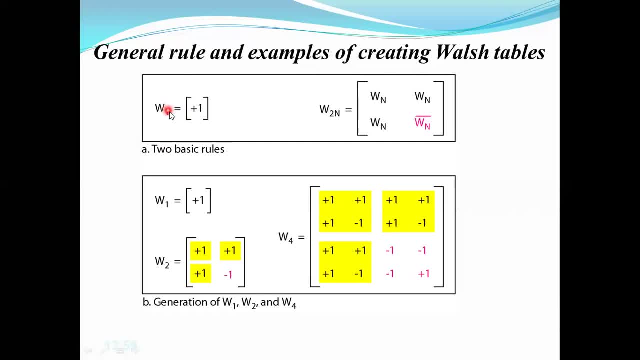 is nothing but one chip sequence. w1 is the default one chip sequence. that means it is having only one row and one column. right, one row and one column here. then w2n is nothing but two chip sequence. w2n is nothing but two chip sequence here two rows as well as. 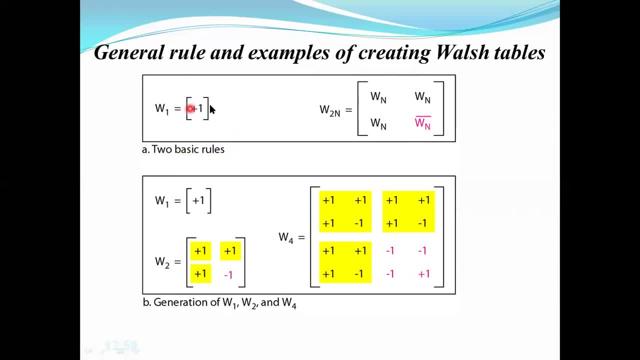 two columns. these are the two basic rules. you need to use it for everything. right now. let us take one of an example: generation of, uh, one chip sequence, two chip sequence and four chip sequence. okay, with the help of this basic rule, we have to generate. we have to generate one chip sequence. 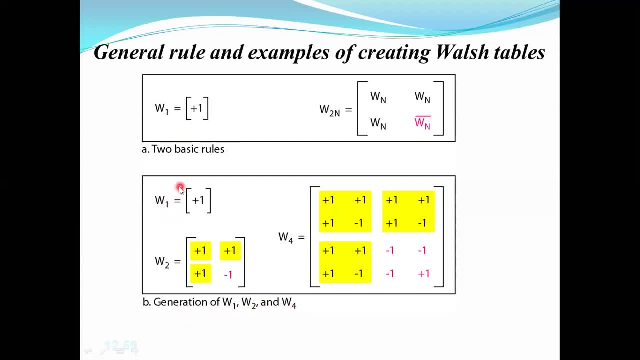 two chip sequence and four chip sequence. this is what the one chip sequence supposed to be. what is that plus one? right see uh here one of the very important things you need to uh note out here. uh, in two chip sequences, what is that wn? this is wn and wn, wn bar. what is the meaning of wn bar? this is actually a complement of. 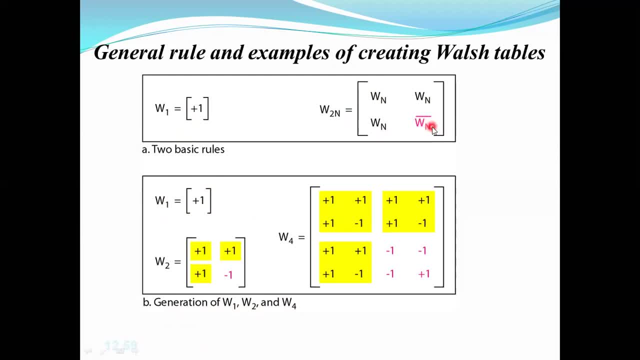 wn right. wn bar is nothing but a complement of wn, complement of wn you are representing as wn bar. this you need to note out here. very important one right in a two chip sequence right: use these basic rules to generate the one chip sequence, two chip sequence and four chip sequence. this is a one chip sequence. this is the plus one, what you've generated here. 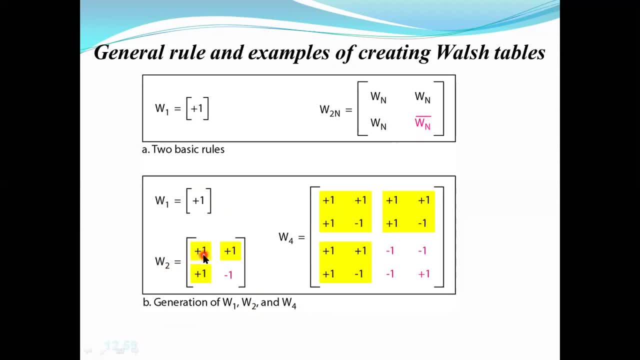 let me come back to the two-chip sequence. two-chip sequence: what happens? wn right. what is the wn value here? wn value is supposed to be plus one right plus one plus one and wn value is plus one. another wn value is the plus one and wn bar. that means complement of wn. what is the complement? 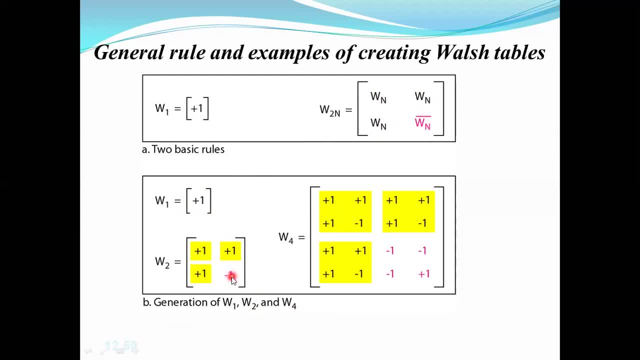 complement of w n plus 1 is become minus 1. that is what the complement of uh, what is the complement of plus 1? complement of plus 1 is equal to minus 1, right, that is how we are representing w n bar right minus 1. this is the two chip sequence. now, uh, this is one of the sequence. you got it plus 1. 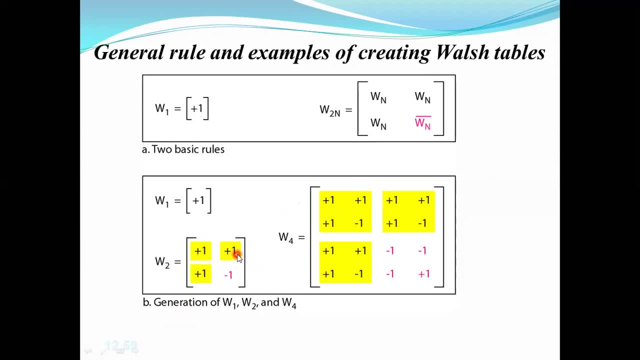 plus 1, the whatever the row you are going to represent, right? this is actually sequence in a two chip sequence. what is the uh sequence supposed to be? plus 1 and plus 1, this is the sequence row. actually, every individual row represents the sequence. right now, let me come. 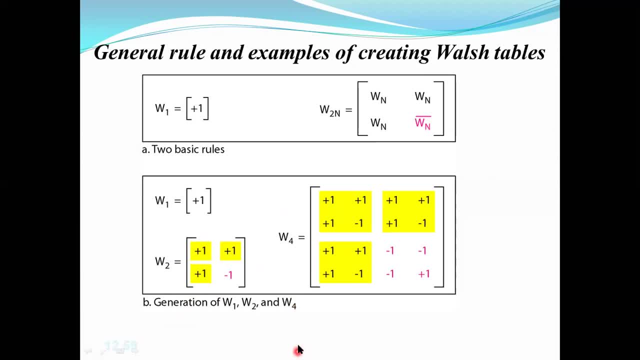 back to the uh four chip sequence here. similar rule will be applied here, or here also four chip sequence. what happens? four rows and four columns. one, two, three, four. right four columns and one, two, three, four, four rows. here now apply the same basic rule here. what is the first one plus one? plus one? 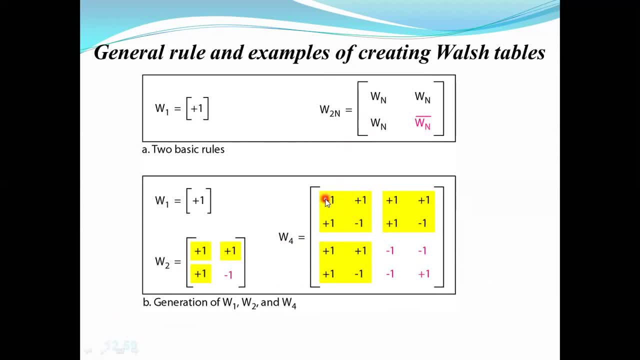 plus one and minus one, right. minus one minus one is supposed to be complement of plus one here. then again next one: plus 1 plus 1 plus 1 minus 1 minus 1 is a complement of plus 1 here. then come back to this: plus 1 plus 1 plus 1 minus 1, complement of plus 1 here. right, use this particular rule only. 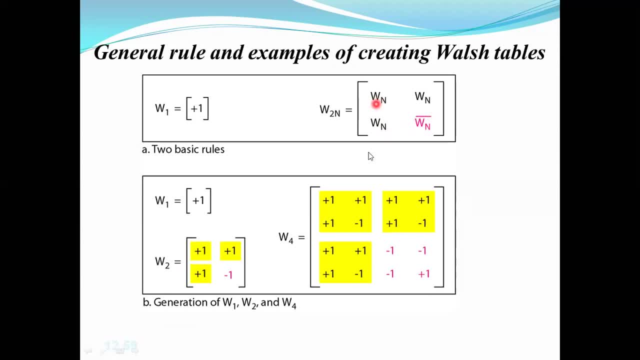 w n w in w? n. what is this? w n bar the complement of wf. now you have to take a complement of this. there's all the values. complement of all these values. this is a complement. right, that is plus one. complement is what? minus one? uh, compliment of plus one is again minus one��, эт ado. Surprisingly, I did not wish to do well without the executor in such a situation when they judge my amateurs to the information in their classines for faculty, to thejan of chemistry, economics to. so I took the leave for Lois with looking at what the teacher said to. 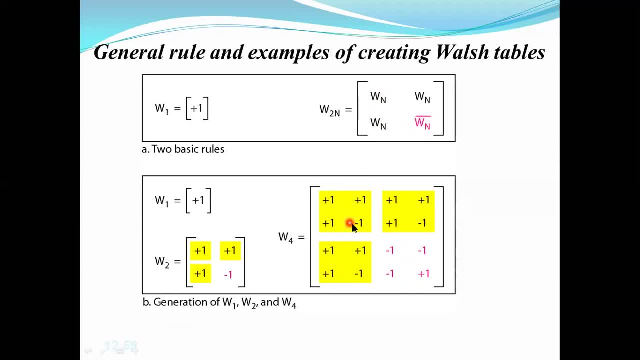 louder from there. what is the discussion there? whether выше or not, the successor in sessions, complement of plus 1 is equal to minus 1. now, minus 1, complement of minus 1 is what? plus 1 right complement of plus? sorry, minus 1 is equal to plus 1. this is what wn bar, this is wn bar. 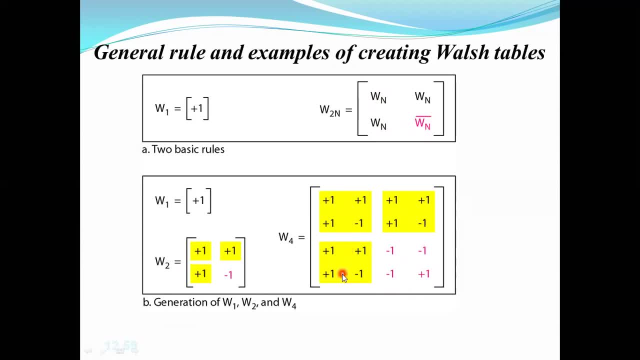 this is wn. wn. this is the wn. now. this is the wn bar. right, you are actually? uh, this case, this is a complement of wn here. this is how you are representing the walsh table. now, with the help of the walsh table, you can easily understand what is the sequence. you can generate the sequence. 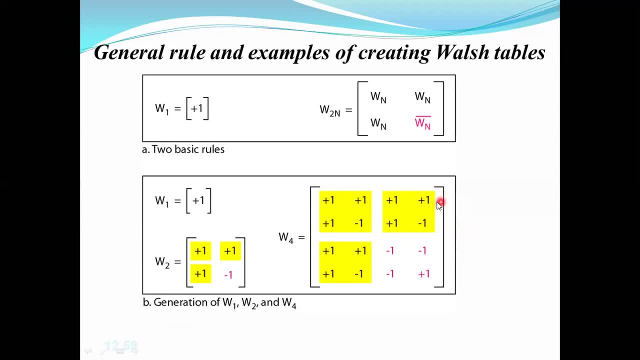